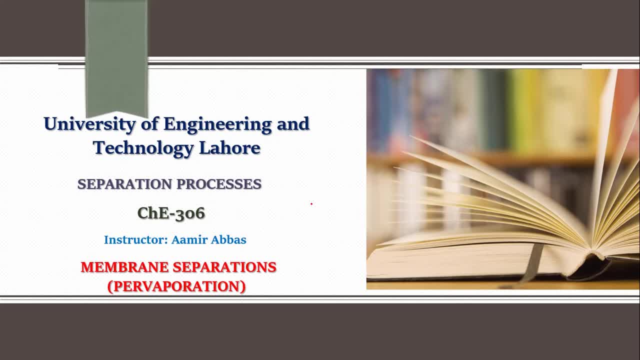 of like size exclusion phenomena. As compared to that, the better is to use dense membrane. And because diffusion or permeability of various gases through various polymeric membranes is different, and based on this phenomena of diffusion difference or permeability difference, you can easily separate various gases. 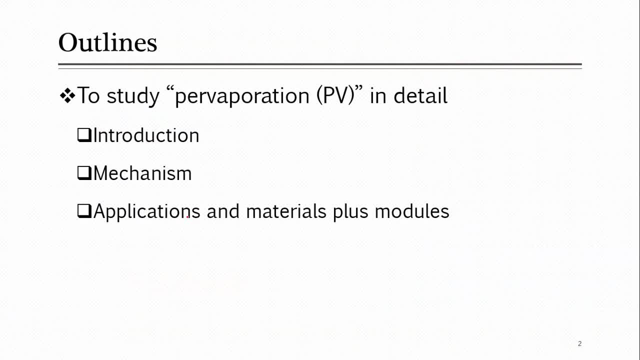 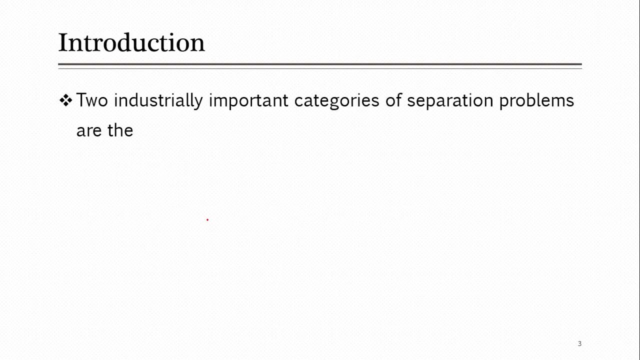 pervaporation. today we have to talk about this in detail, and this will include the introduction, then mechanism, how pervaporation takes place, and then, finally, applications: membrane plus modules used in this membrane phenomena. Let us start with the need for this mean pervaporation. why we go for pervaporation, Actually there. 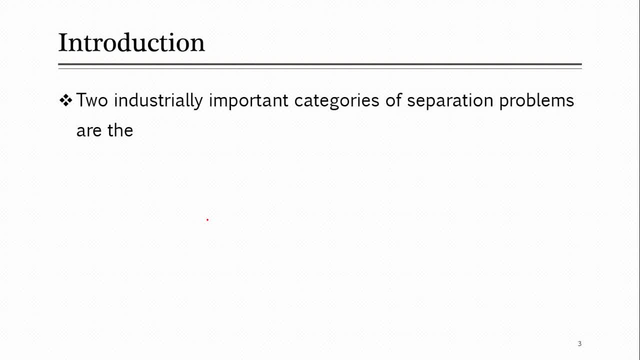 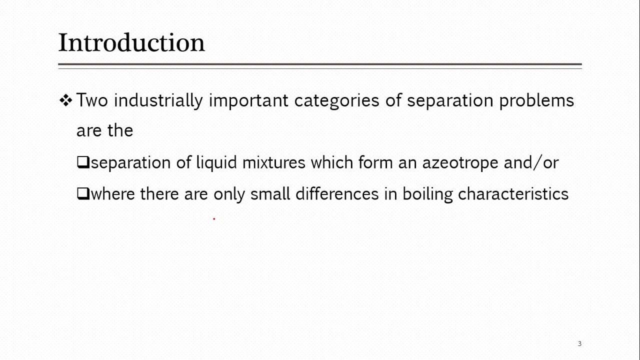 are two important categories of separating various mean hydrocarbons or various components and those separations are difficult. What are those separation? These are two separation like if you are separating azeotropic mean liquids or the mixture where azeotrope is formed. you know that it is very difficult to separate them. I mean when azeotrope is. 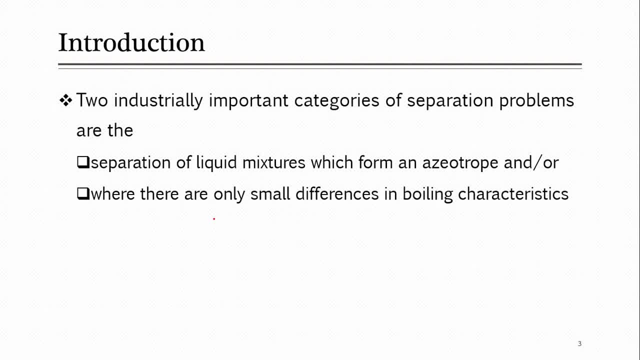 formed, you cannot go for distillation, then you look for other form of distillation. So these are techniques and maybe you can go for like liquid-liquid extraction or absorption. but we, when we started the membrane, we said that membrane are better as compared to those. 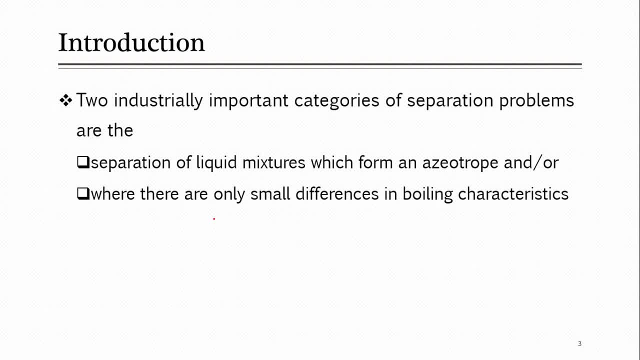 other separation technologies due to various advantage which we discussed at the start of membrane, when we started with the membrane. that why these are better as compared to other techniques, Although you can separate these azeotrope with the help of maybe liquid-liquid extraction or maybe absorption. 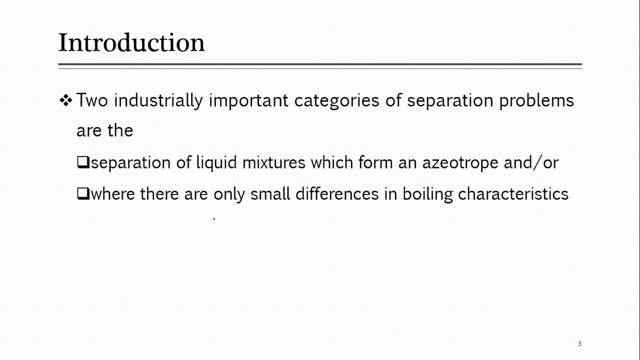 Thank you very much, But membrane separation will be better for such kind of separation. The other are when there are very small differences in the boiling characteristics. Again, you know that it is difficult to separate them with the help of distillation, because when their boiling points, 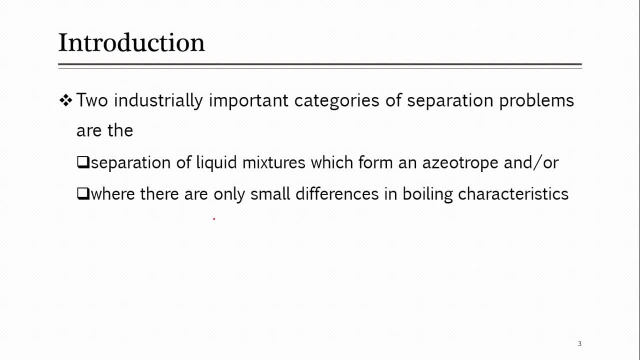 are closed and their volatility differences are very small, so it is not possible to separate them, Although you can separate them, but you will need very large size equipments and energy consumption is way higher as compared to simple separation. So mean in these cases. 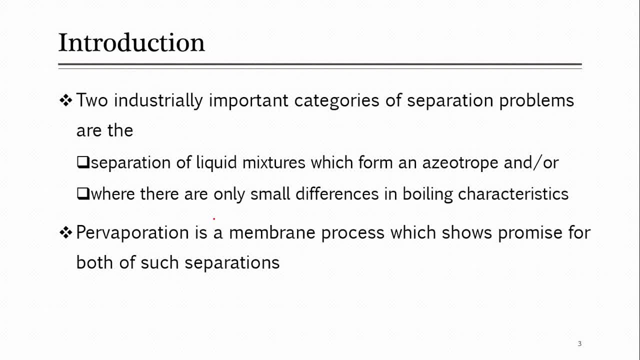 per-vaporation phenomena can be used or per-vaporation membranes are used for these separations And, by the way, this mixture. both mean- this is the liquid mixture- and again, which have small difference in boiling. what does this mean? it is mean they will also exist in the liquid form. So overall you can say that this per-vaporation use are through water. telephone you may be using something called water And then that is when the spine has some of its makeup and it means that it is there and that they are collected and stored. 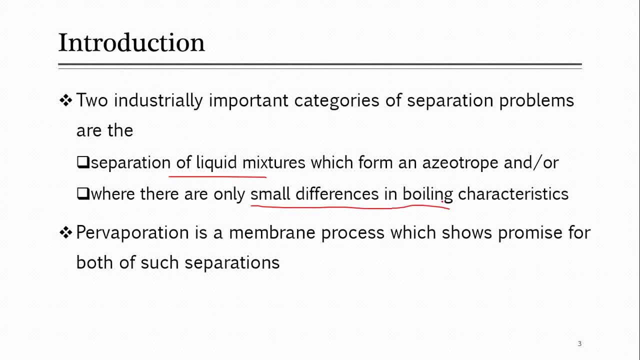 on the surface At first, this lesion is really difficult Also. this겠죠 narrows down, so the technique is used for separation of the liquids. As compared to this, like gas separation, that also can be used for, like these, hydrocarbon or other gases separation, but they exist in. 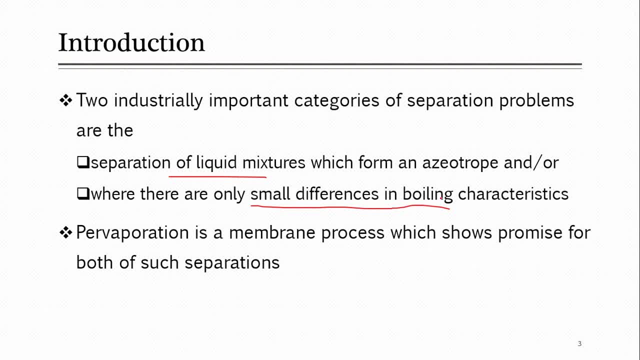 the form of gases. like RO was for water, then gas separation can be used for any mixture of gases and this pervaporation is used mostly for the separation of the liquids and, most of the time, its application. we will discuss later on in this lecture that it is for hydrocarbon. 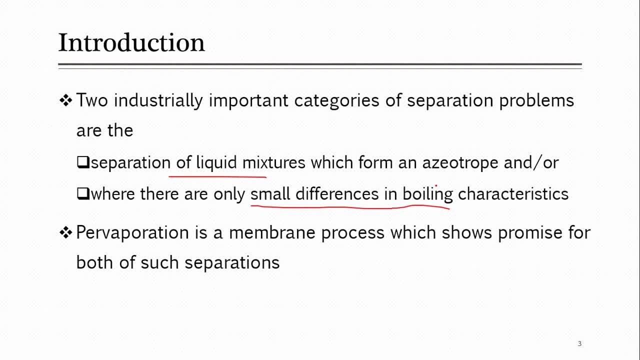 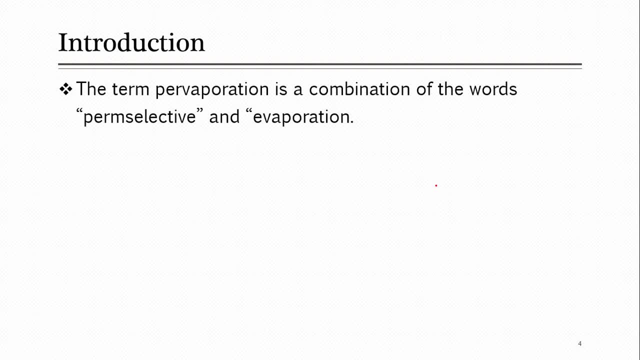 separation and when they exist, actually in the form of liquid mixture. So pervaporation is the best way to separate them. So its name like this: pervaporation. this is combination of two words: pump, selective, and then there is evaporation. So if you just take from here per and then just evaporation, 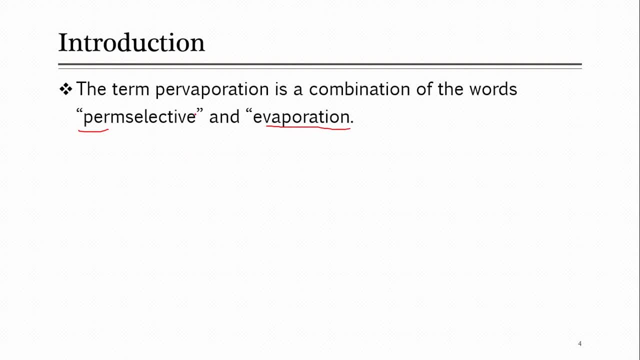 So pervaporation is the combination of this. what does this mean? pump selective membrane mean you know that this is type of membrane in which we have a like asymmetric membrane, and that consist of more than one layers, like there can be dense as well as porous membrane. 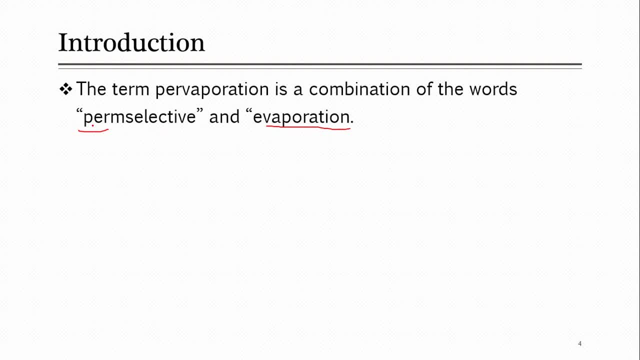 structure. it is a combined structured membrane or you can say its composite type membrane. and then there is evaporation. I mean you are just, And you are just evaporating anything which is in the form of liquid to the vapor. So in this technology, when you will be using the membrane, actually with the help of this, 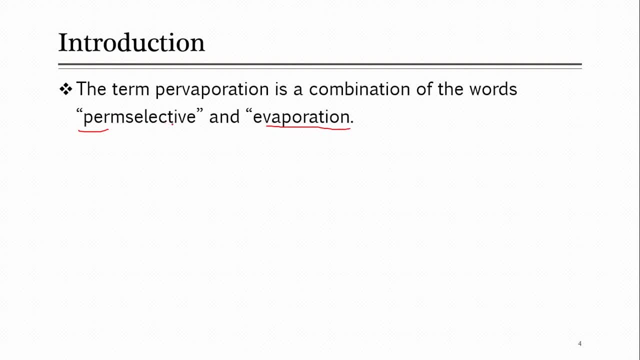 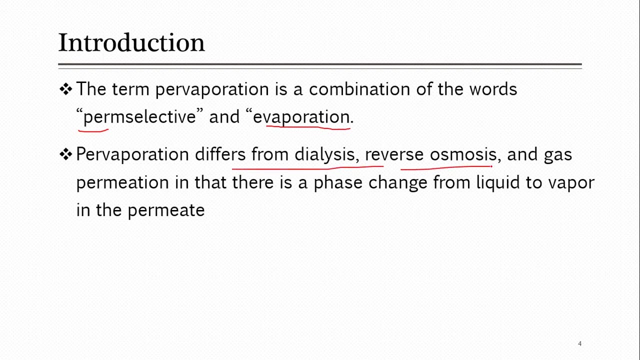 pump, selective membrane. You are making the separation. at the same time you are change, you will be changing the phase of those components which are being separated. So this technique will involve actually this differ from other life techniques which we discussed here: reverse osmosis and 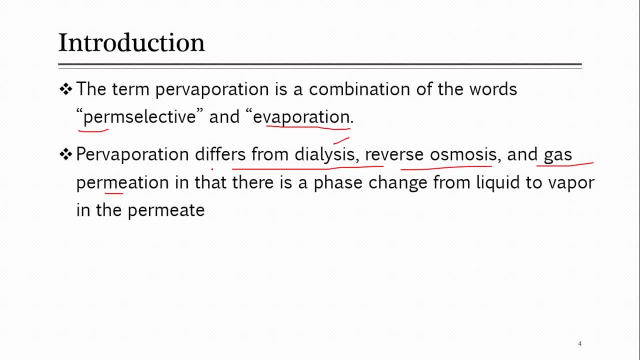 gas permeation, dialysis, which was not included here in our main subject, but at those, all type of membrane when you will use for these application, like dialysis, reverse osmosis or gas permeation, there were no phase change involved, At least you remember from reverse osmosis and gas. 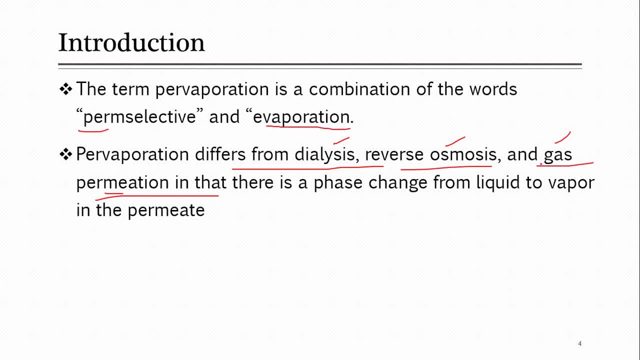 separation or gas permeation, which we have discussed- that when you were using these membranes, at least there were no phase change In the case of water. you remember that when water pass through this membrane, that remains in the form of liquid As well, when gases were. 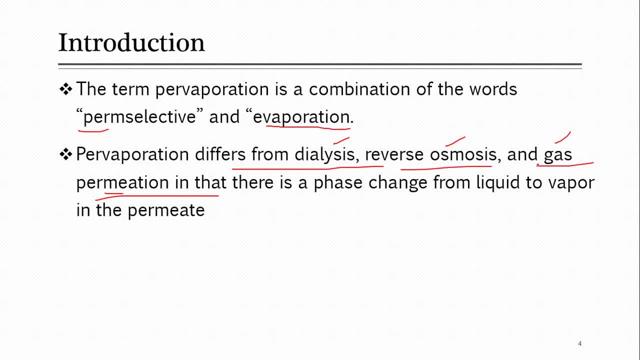 passing through the membrane. they were supposed to stay in the form of gas, and they stay in the form of gas. they did not get condensed. But in this technique- power evaporation- there will be phase change. How phase change will take place, we will look at this later. but 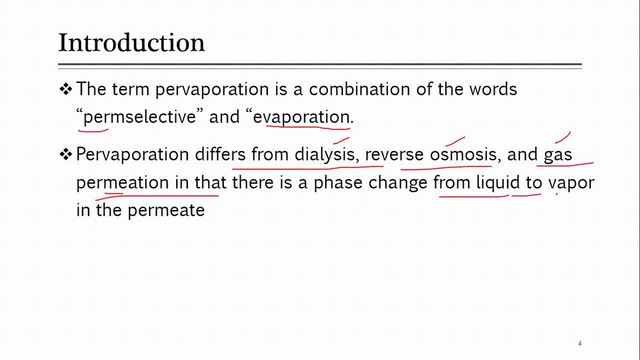 at this moment. So at least its feed is in the form of liquid, but on permeate side it is converted to the vapor. I mean all those component which pass through the membrane are permeated and as collected, as permeate, they are in the form of vapor, While other, like its feed, exist. 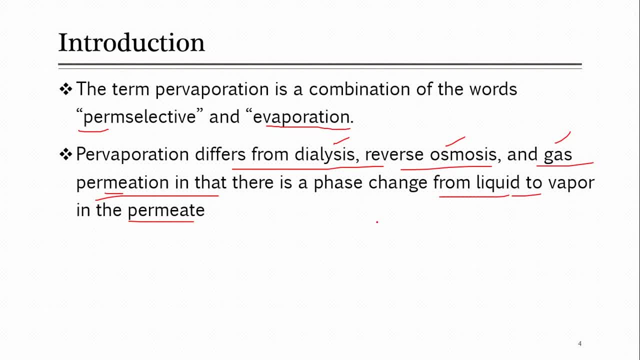 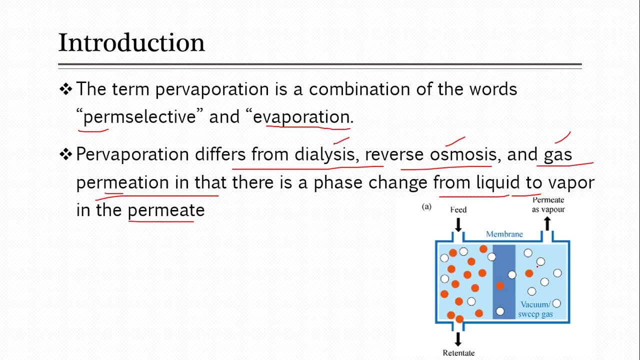 in the form of liquid and retentate will also be leaving in the form of liquid, For example, here in this cell. you can see that this is one cell on which There, in this, on this side, there is feed and then membrane is installed inside this And 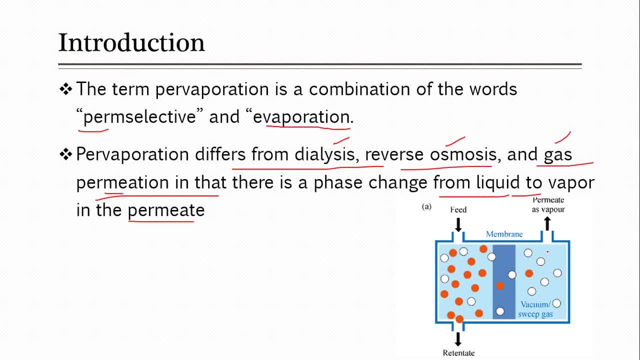 on the other hand, you are collecting like permeate, because here is mentioned one, However, we mentioned here somehow vacuum is applied on this side And when you are applying the vacuum, some component of it can pass through the membrane, like these white color dots. These components can easily pass through the membrane or there are good permeability if 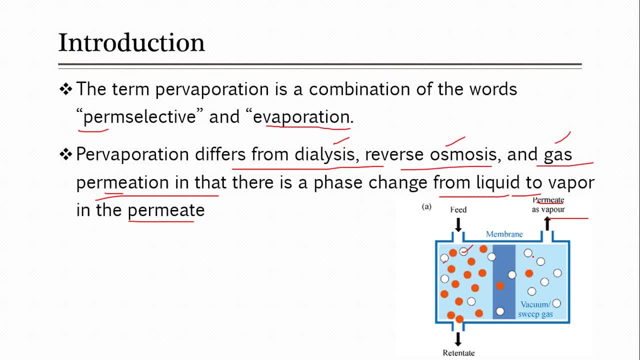 there is a few other as opposed to it. As so, the membrane is working instead of naturals permeability as compared to this. So when they get separated, they reach to the other side of the membrane, they are evaporated, they are converted to the vapors. 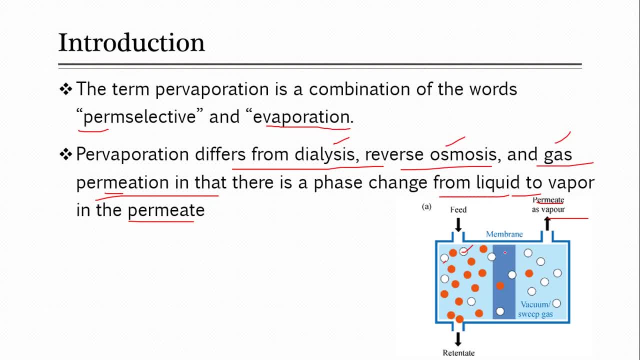 And later I will talk why we go for ROK. just with- let us discuss it here. few lectures back, if you remember, we discussed the comparison between- I think that was some starting lecture of membrane separation. So we discussed there like if you are using the membrane and various 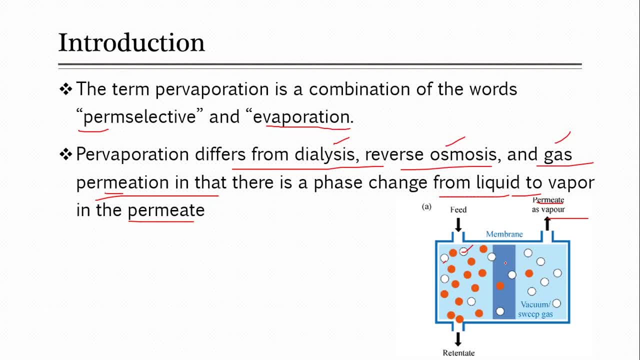 diffusion of various species. actually we were comparing those like. there is diffusion of solid, diffusion of liquids and diffusion of gasses through the membrane. So, if you recall, diffusion of gasses was the highest. or if something, when is existing in the form of vapors or gasses that can easily diffuse through the membrane, or their diffusion was. 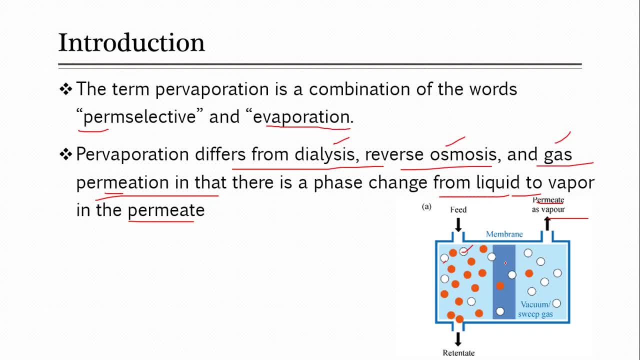 fast. There was comparison between, I think, molecules of water which were passing in the form of either solid liquid or vapor through various membrane components, So their diffusion was different and highest diffusion was possible when they were existing in the form of gas. So here, when some species just 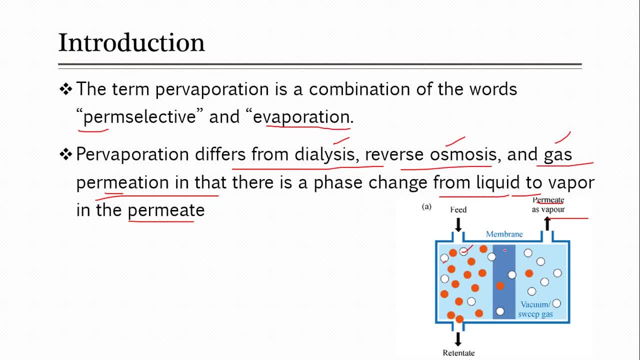 pass through this membrane and if it is converted in the form of vapor inside the membrane, so its diffusion will increase And when its diffusion is increasing, definitely its mean separation is higher as compared to other component which will diffuse like slowly Overall. with this I mean you are increasing the rate of diffusion, rate of separation. 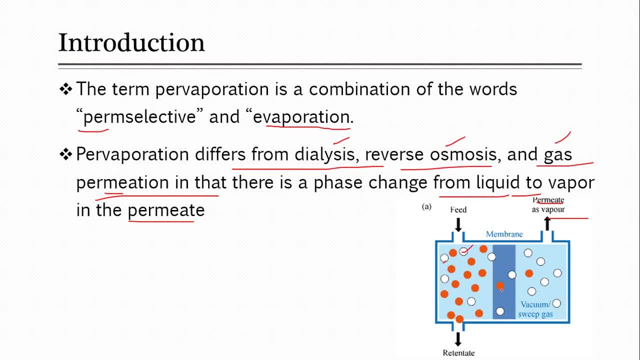 when you are using pump selective membrane. Hopefully it is clear to you. So again, we will discuss this point later on in the lecture. But the major purpose here, pervaporation- is to Evaporate the species which are diffusing through the membrane. and when we are just 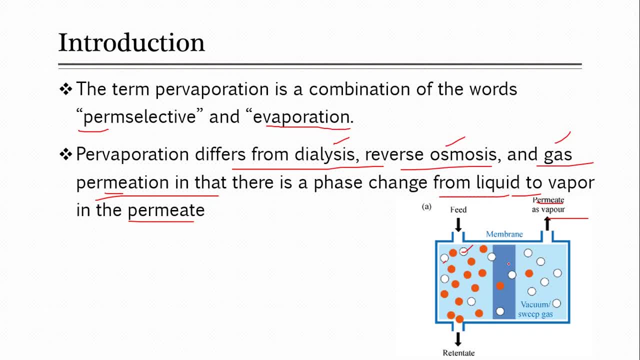 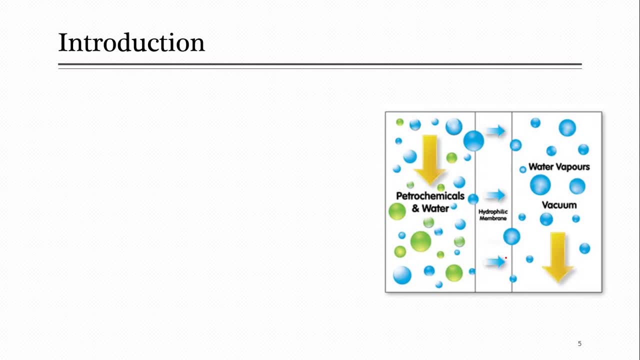 mean evaporating. with the help of this, actually, you are increasing the rate of their diffusion and mean separation through the membrane. Here you can see another like system in which you have a mixture of various petrochemical and water molecule and there is a membrane here, And this membrane is hydrophilic membrane. So hydrophilic, which is which attracts the 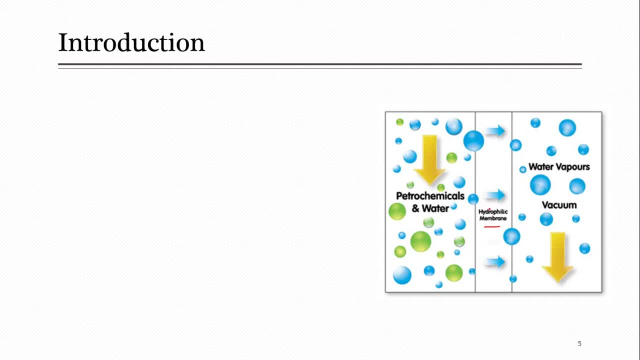 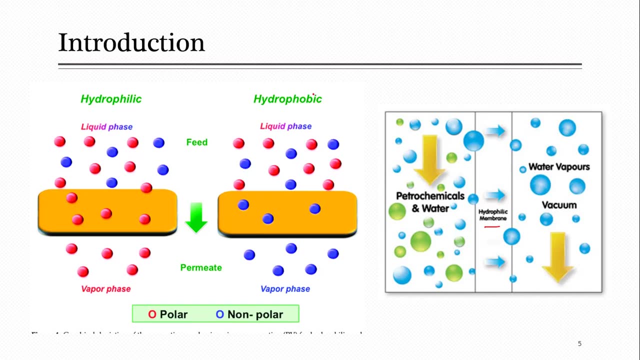 water. I mean hydrophilic, which has affinity for the water, and there is other term that is called hydrophobic. So they mean they repel the water. They are not water loving. This hydrophilic will attract the water, and when mean they have good separation capability. 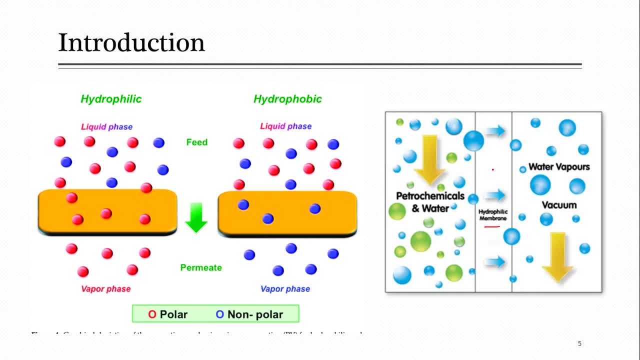 for the water, or water can easily diffuse through this membrane. So when you are using this membrane on the other side, when water is water, vapors are oger which may separately excited this membrane, getting harm. so we will just see When we are using the defence mentre in the rebound, So vapors are also. did they move? 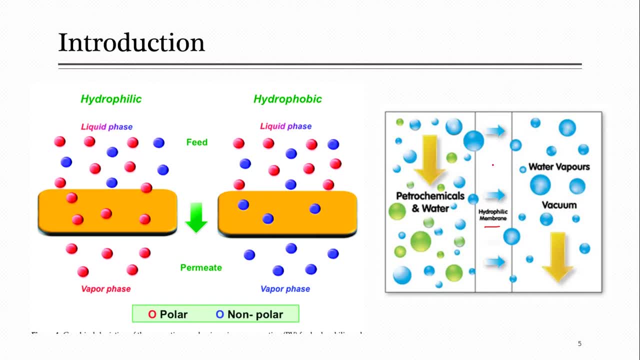 to the tuber a true liquid. That is very important science and, by the way, why we are going to a nice one. Okay, and, by the way, this mean how it this evaporation take place? because something is in the form of liquid is on the one side of membrane And when it pass through membrane, 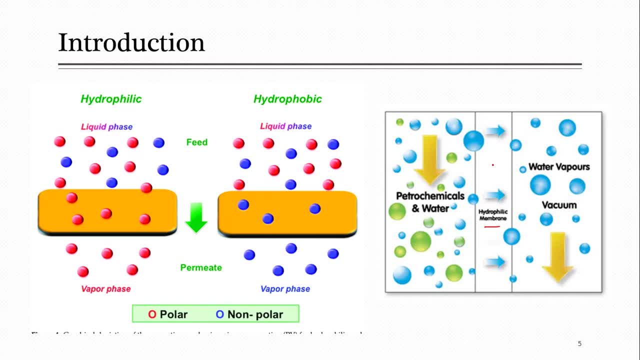 how it gets converted to the vapor. So we apply actually the vacuum on the other side And when you are applying the vacuum actually you are decreasing the pressure on the other side of membrane And because in order to convert something from vapor to the liquid, 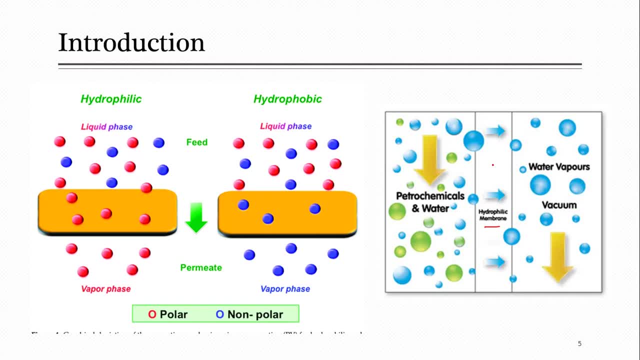 sorry, liquid to the vapor- Slide 31. all the other fact solve is there? yes, Slide 31. Well, all data for evaporation are existing in the diagram, but it is absolutely stressed with the to the vapour. you just go either for heating when you increase its temperature and when 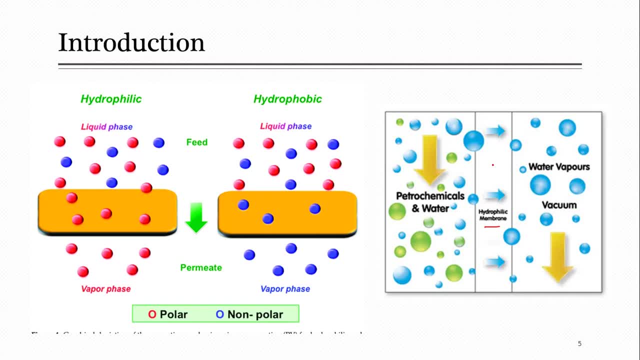 its vapour pressure reach or becomes equal to the surrounding pressure or ambient pressure, then its vapours are formed. Now here we are. when we are decreasing the pressure, we are creating the vacuum due to this. when you are decreasing the pressure, you are decreasing the surrounding or ambient 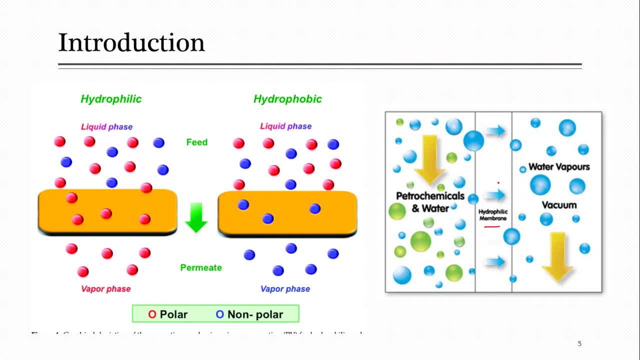 pressure, and when ambient pressure is reduced, their boiling point is reduced and they can easily boil, even at low temperature. due to this, they are converted to the vapour, For example here, if we are considering the water, if it was ambient temperature, ambient pressure on this side. so for this you will need temperature of 100 degree C, but when 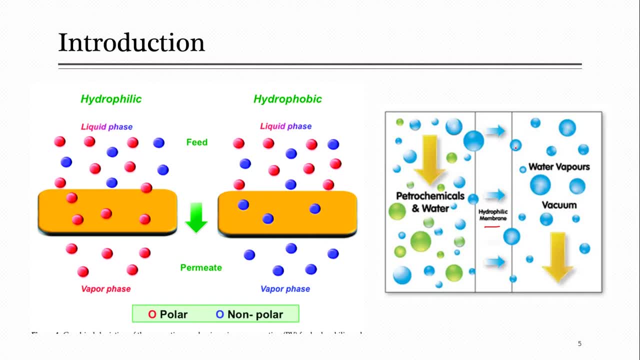 you reduce it definitely. it can boil easily, even at temperature which is below 100. This, This membrane- here I mean there are two phenomena- shows to you like there are hydrophobic and hydrophilic membrane, when you, when you are going for these separation by using pervaporation. 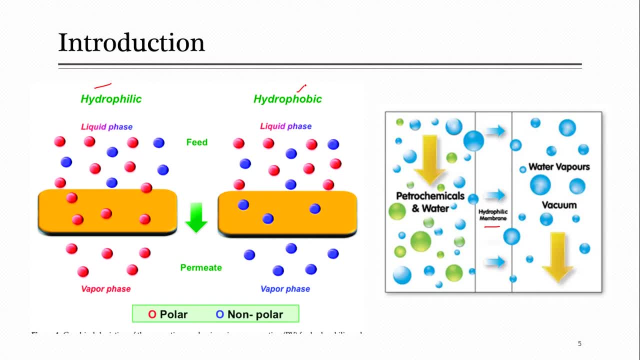 later on you will look at the application that a lot of application of this pervaporation membrane is for removal of water through removal of water from various hydrocarbons. So if you use such membrane which is water loving or hydrophilic, so in that case water 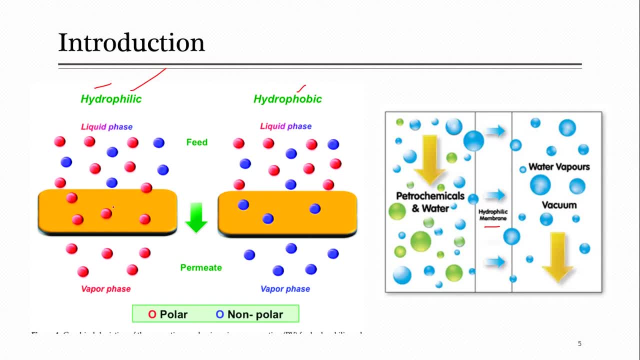 will Easily diffuse through that membrane and can get separated, while on the other hand, if you are using the membrane which repel the water, so in that case that membrane should have affinity for other component instead of water. for example, water is in large amount and some other hydrocarbon are in very small amount, so we will prefer to just pass those. 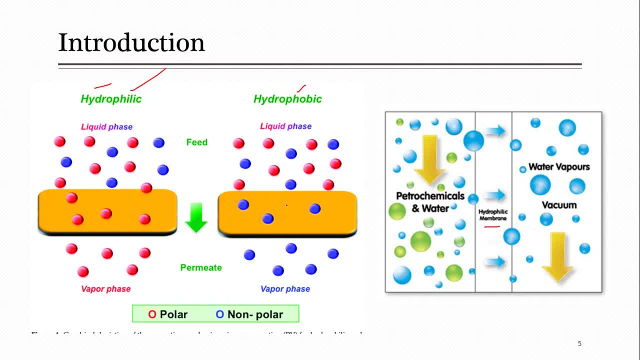 hydrocarbon through the membrane and can get them separated. but if hydrocarbon are in large amount as compared to water, So In that case we will prefer to remove water through this membrane. so in that case the those membrane will be used at like hydrophobic if you want to repel the water away from the. 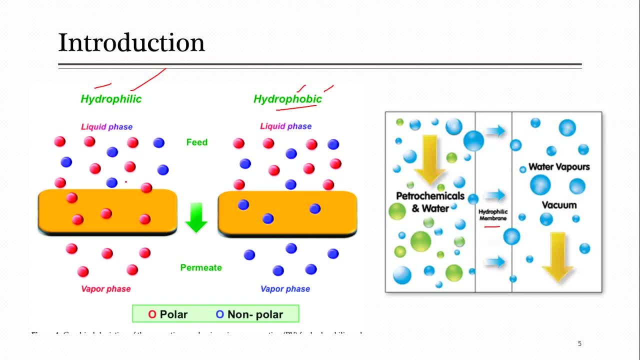 membrane. but if you want to pass water through the membrane, so then you will prefer the membrane which has affinity for the water. so in these both cases, actually feed enter, pass through the membrane and on the other side they are converted to the vapor. again same, like phenomena. 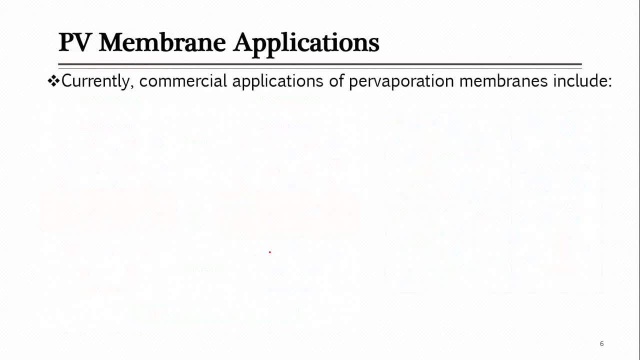 here you will be applying Vecume, Vecum, Vecume, Vecume, Vecume, Vecume membrane. this PV stand for this pervaporation membrane and these pervaporation membrane are used for actually right pervaporation membrane application. 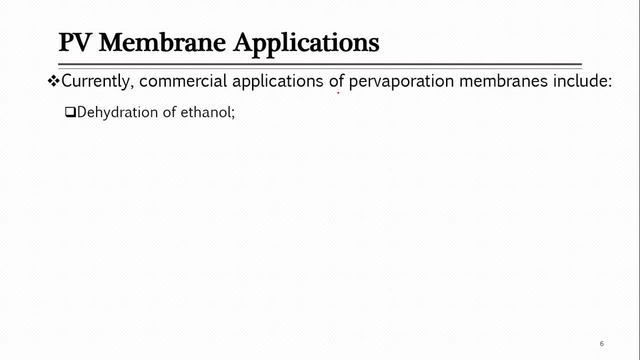 These currently commercial application of pervaporation membrane include a dehydration of ethanol, If you have to remove The water from ethanol. when water ethanol is produced and this it also contains water. So in order to remove water from ethanol, these pervaporation membrane are the best available technique. 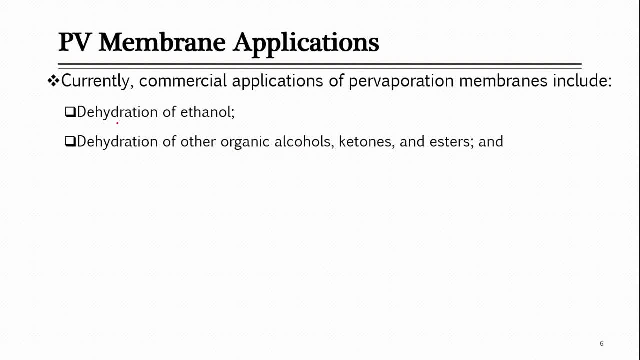 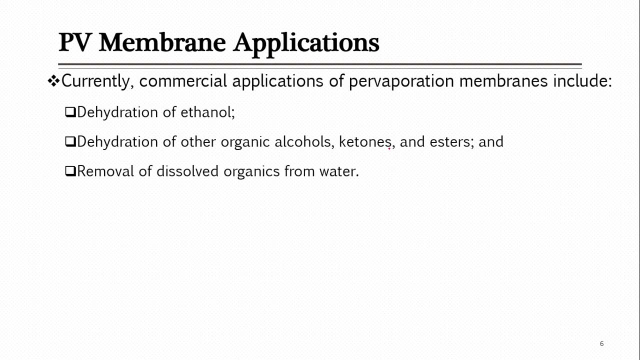 Then there is dehydration of other organic alcohol. this is ethanol mean. if suppose you have propanol, methanol, ketones esters, So also water can be removed from those main hydrocarbons. and then there is removal of dissolved organics from water. I mean in this: 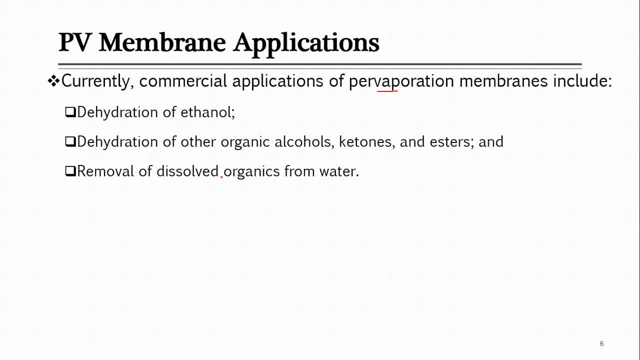 application. water is in large amount. if other, some small amount of hydrocarbons is there, organics are there along with water, So those can be removed with the help of this pervaporation membrane. If you remember when we discussed liquid-liquid extraction- in that there was at the start of that lecture- there was some application. 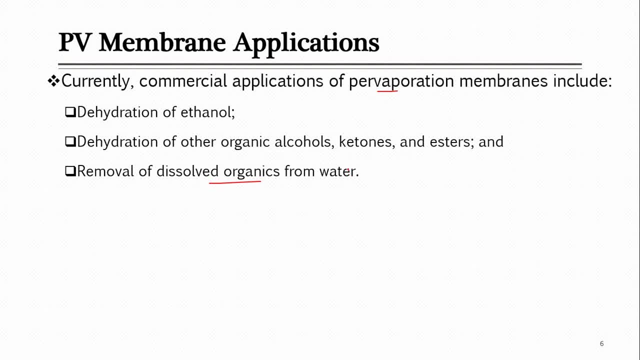 of this liquid-liquid extraction. So there was some application of this liquid-liquid extraction in that there was at the start of that lecture. there was some application of this liquid-liquid extraction for removal of water from acetic acid. So in such case, 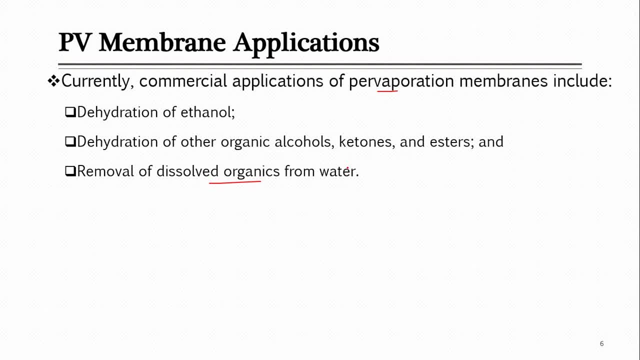 like, you can either use that liquid-liquid extraction or membrane. but as you have studied now that membrane are better as compared to all those techniques because they are compact, they cost less as compared to other technique, the equipment are smaller in size, they are easy to install and various other advantage. I mean give. I mean they can. membrane can be. 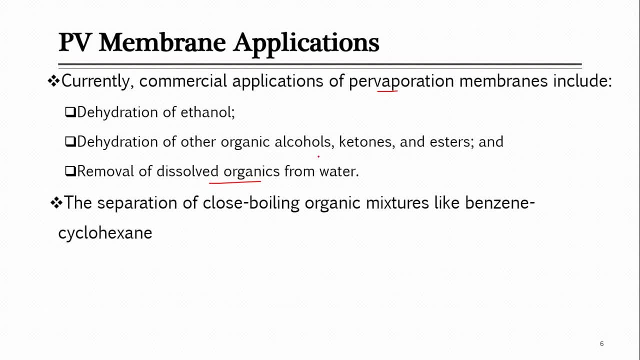 preferred as compared to other techniques. The separation of close boiling mixture. you know that it is again I mean difficult to separate them. the major point. at the start we also discussed that close boiling organic chemical are difficult to separate. So for those application this pervaporation membrane. 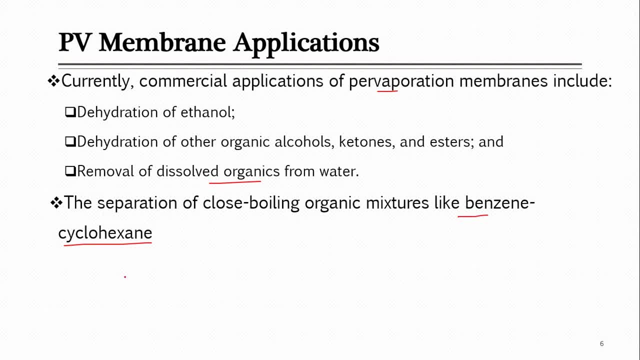 are good, and because this now benzene and cyclohexane, they will be close to each other, also be close diameter of the mean molecule as well. their boiling points are close to each other. So in this case means you cannot go for distillation, then it is better to look for other technique. 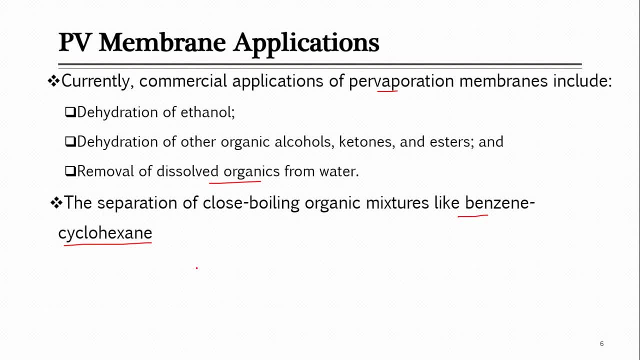 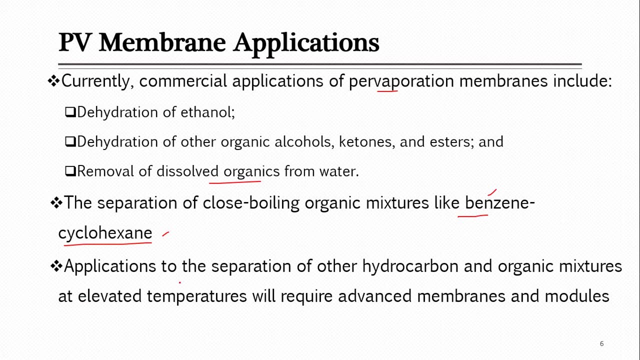 and among other, when this membrane separation is good. So you can separate this mixture of benzene and cyclohexane by using these membranes. So their application to separation of other hydrocarbons- So many hydrocarbons some- some difficult separation may be if they are existing. they. 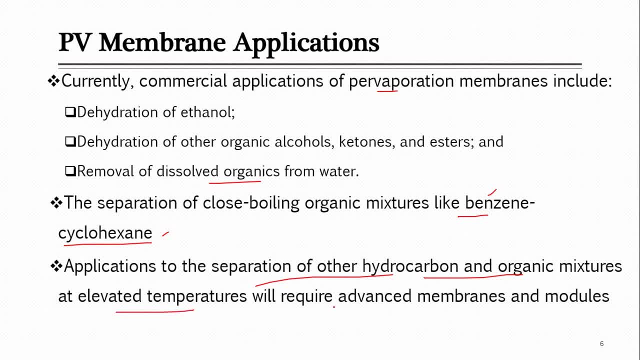 are a huge mixture and they are at elevated temperature mean they are available at high temperature. So their separation- you know when temperature as high then mean polymeric membranes- are not that good. you have to use some other membranes which can separate them and those are inorganic membrane and those advanced membrane mean inorganic membranes. 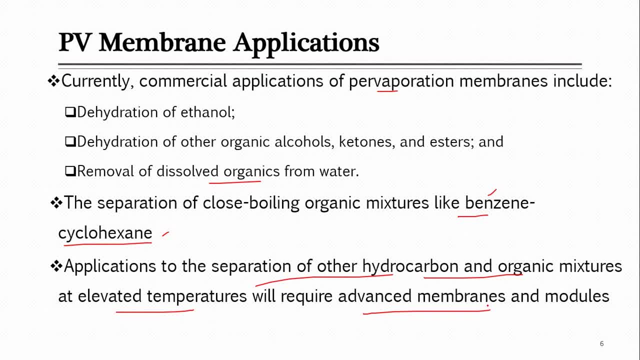 can be used be organic, inorganic, composite membranes which can exist or which can perform separation at high temperature. they can be used for such kind of separation. But at the end, just to conclude, these application main membranes, pervaporation membrane, have found a lot of applications on industrial scale for various separation of majorly closely. 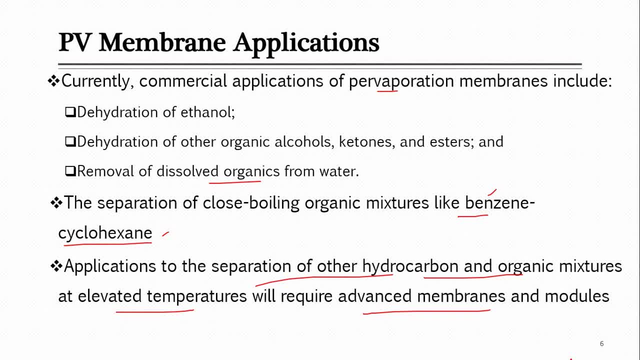 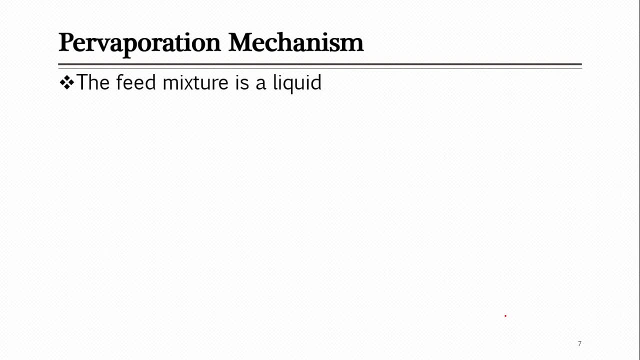 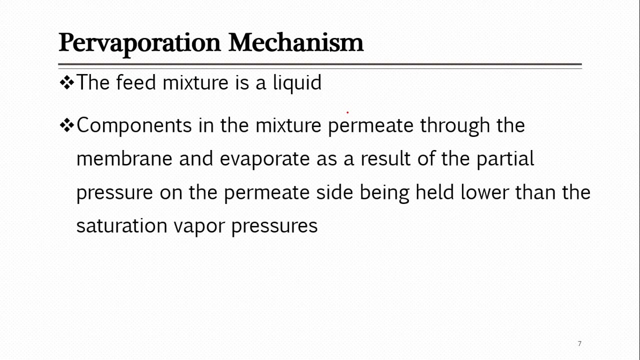 boiling hydrocarbon, as well as to remove water from various hydrocarbons mixtures. Let us look at the mechanism. how does it take place? So somehow we have discussed few points before this, but overall you know that feed mixture here is liquid. mean feed entering to this system is liquid. 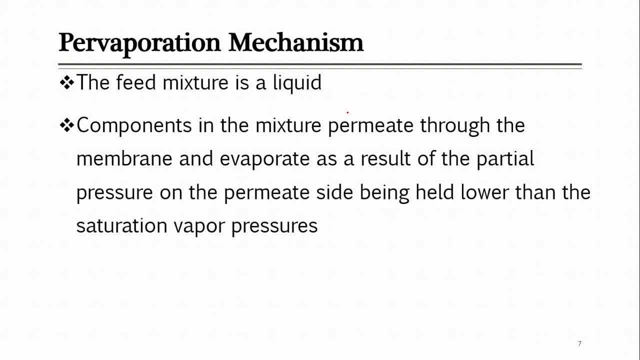 Then some components in this feed, in this mixture, can permeate through the membrane and they are evaporated Mean on the other side of the membrane. when they reach to the other side of membrane, they get evaporated. actually, they evaporate as a result of- I mean partial pressure on the 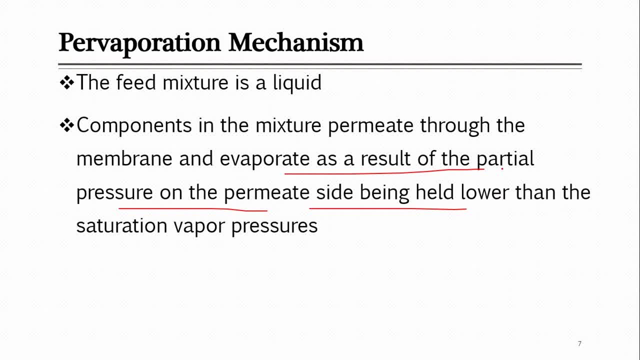 permeate side being lower They are suppose. if mixture is just passing through this, then you will look at the partial pressure. if out of mixture only one component is passing, then we will say its mean boiling temperature or its saturation temperature. But if 2 or 3 component, 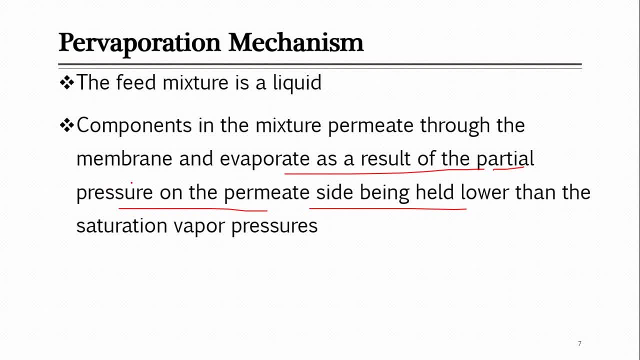 Of course, Of course, Of course component can diffuse through the membrane. So definitely, then you will be looking at partial pressure of each component. So they are, at the end, actually lower than the saturation. sorry, their surrounding temperature is lower than the saturation pressure. surrounding pressure: 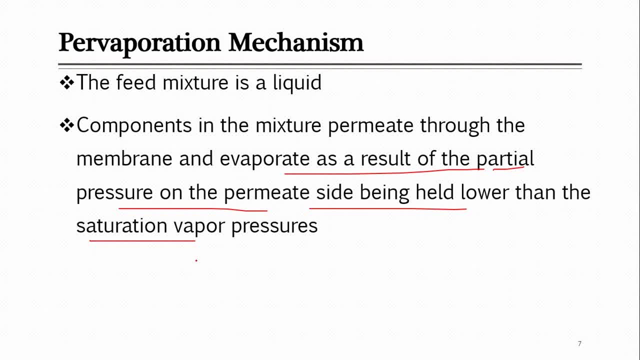 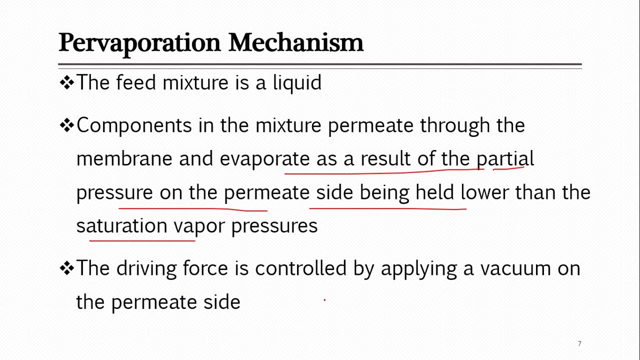 when will be lower than due to this vacuum. due to this low pressure, evaporation take place and their phase is converted to from liquid to the vapour. The driving force is controlled by applying the vacuum here driving force. we discuss this. the driving force for reverse osmosis was the pressure, high pressure, on the feed side. 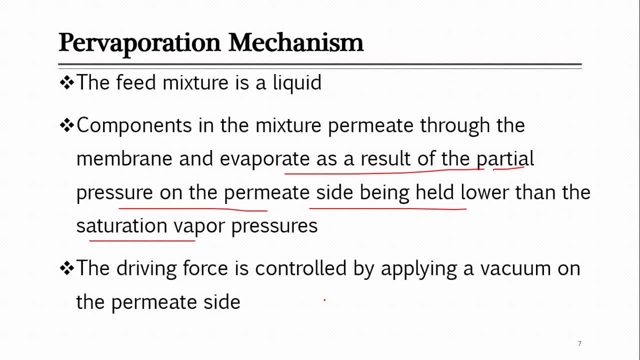 and low pressure on the permeate side as well. For the gas separation very high pressure was being used on the feed side and low like almost ambient temperature was used on the gas side, on the permeate side. but in these membrane mean you mostly bring the liquid at not very. 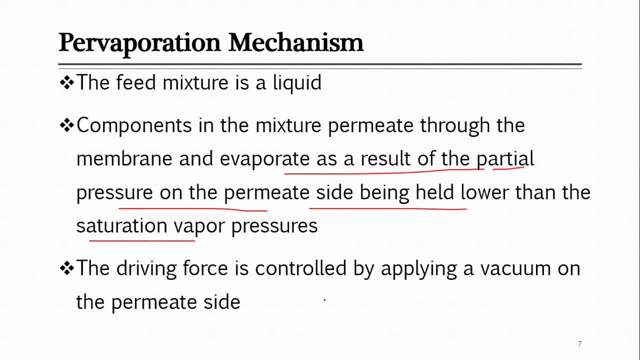 high pressure sufficiently. high pressure mean like, not like the pressure which we discussed earlier. like in gas separation membrane, if you remember. it can vary from somehow 10 atmospheric to 150 atmospheric on feed side. So here mean you bring those usually at low pressure. 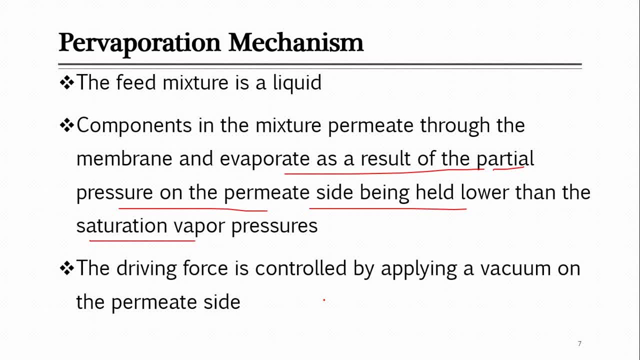 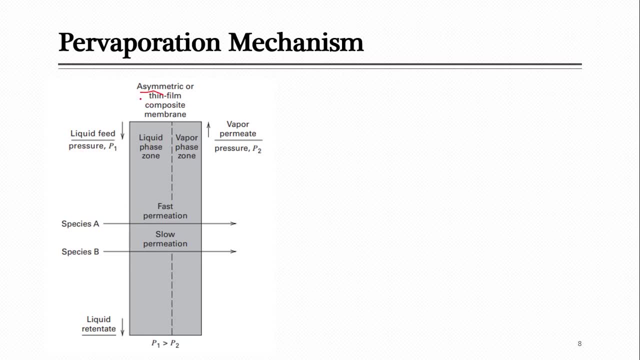 but on the permeate side, actually you are providing the vacuum. So now, when you are providing the vacuum, definitely you are creating the pressure difference here. So with the help of that, this separation take place. So let us look at this membrane. it is again asymmetric membrane. most of the time we are 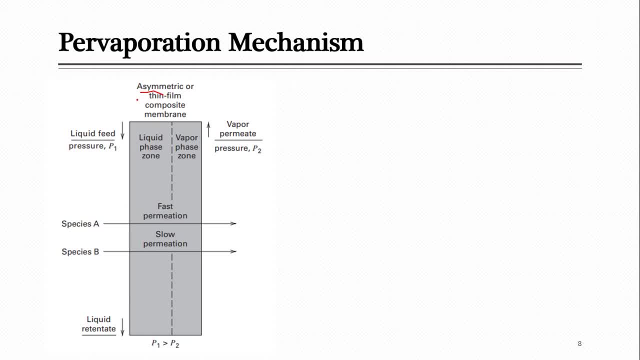 using asymmetric membrane for all application which we have studied: reverse osmosis, gas permeation, and again, this is again asymmetric membrane And the phenomena is: this is the same, or the reason is the same to use asymmetric membrane? because you have to apply the pressure difference on the both sides of membrane and it is not possible for the dense membrane. 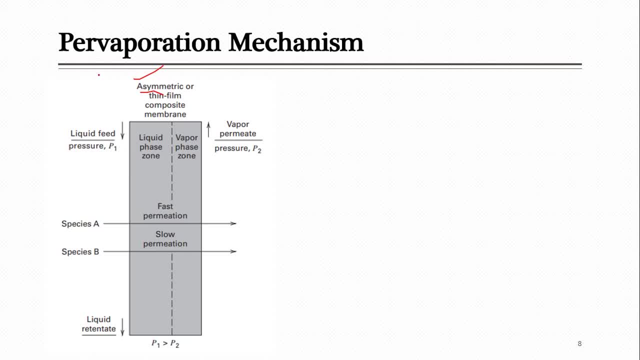 simply one sheet to support that high pressure, Otherwise it is, rupture will take place and in order to avoid that rupturing, you are using asymmetric membrane. So they are like combination of porous and non-porous membrane. at the top there would be non-porous layer or dense layer, which is mainly for separation, and then there are porous. 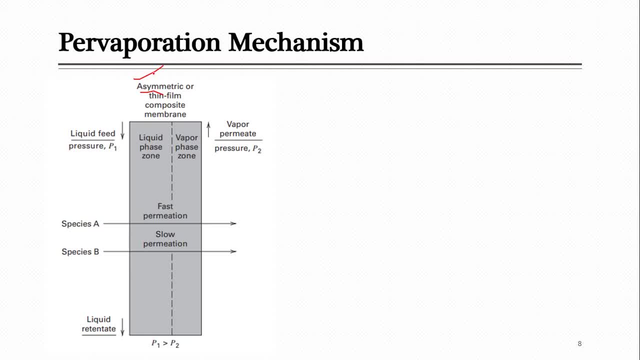 layers. Sometime one layer, sometime two layers are possible. I mean then it is asymmetric membrane and they are used for supporting the membrane On the one side, I mean feed side. you have a liquid feed and it is available at pressure P 1 and that consist of two species, A and B- Just look here like feed to the membrane. 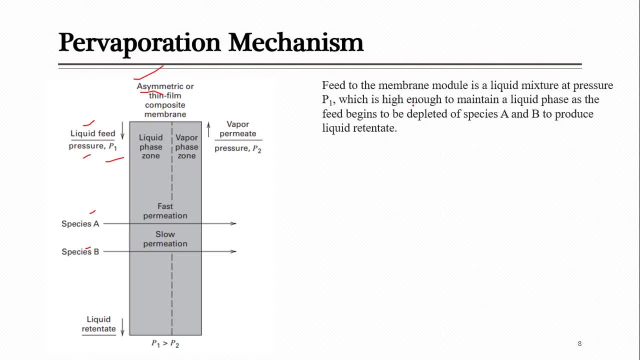 module is a liquid mixture which is at pressure P 1 that is high enough to maintain a liquid phase. So here pressure should be high enough that you can maintain a liquid phase. I mean it did not get vaporized on this side of membrane, feed side vaporization should not take place. 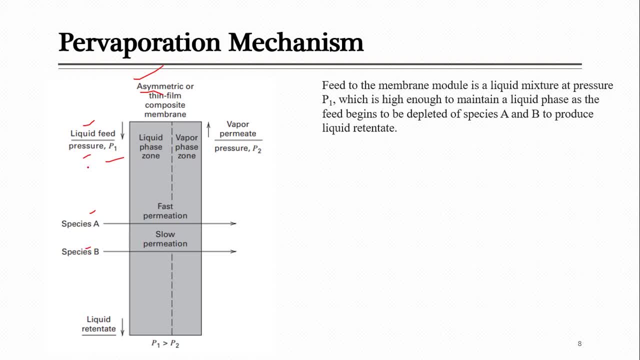 Pressure should be sufficiently high that all the components which are available as the feed they stay as a liquid when this exist on the feed side, And I mean even when some components are removed through this, like A and B Component, when feed enters from this part and it is going through this membrane and 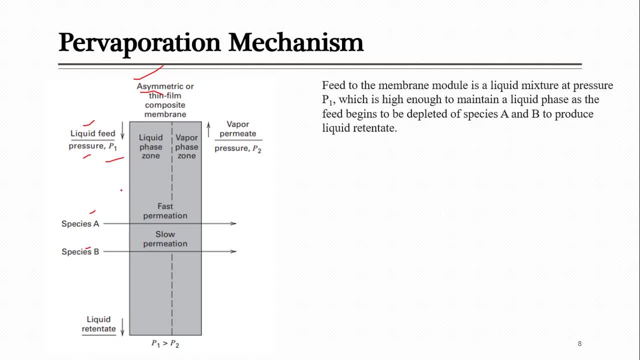 and the other and it leaves. but when it is passing along the membrane, some component definitely will diffuse through the membrane which are like A and some part of the B, As you have seen here. he has mentioned that fast pervaporation. it is means, sorry, fast permeation. 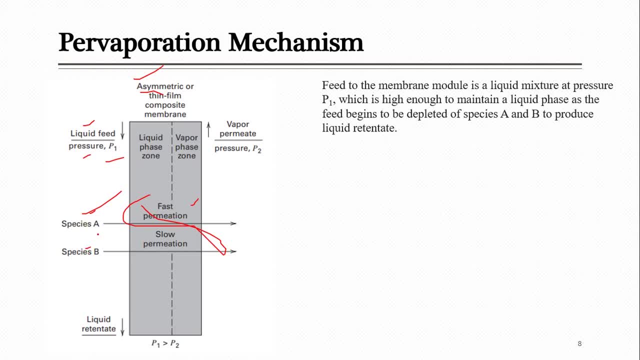 So component A, if you are considering A and B, just two components. So component A has fast permeation. it is mean majorly A will get diffuse through the membrane and it is separation takes place. So component A will get diffused through the membrane and 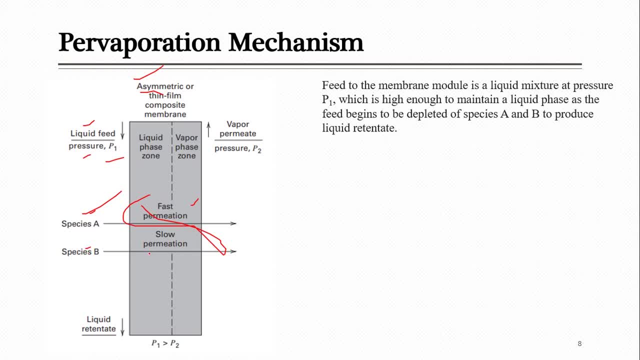 it is, separation takes place from B, While, as already you know, that membranes are not like 100 percent selective for one component. some part of the B will also diffuse through this membrane, But it is a permeation is very slow, as in the first diagram we have seen. 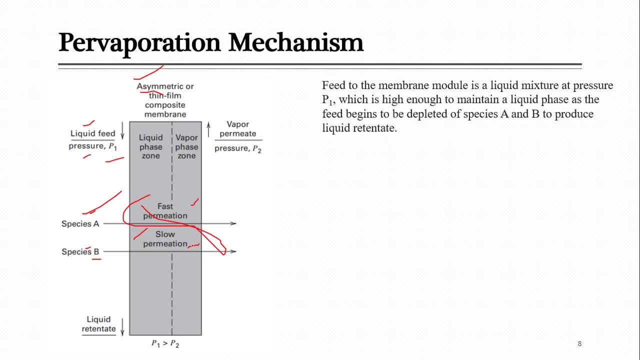 there were some red and white circles, and white circle parts can diffuse in the large amount as compared to other which were in the form of red. So this also will pass through, but small amount will pass through. So even when this membrane is not like 100 percent selective, for one component, some part. 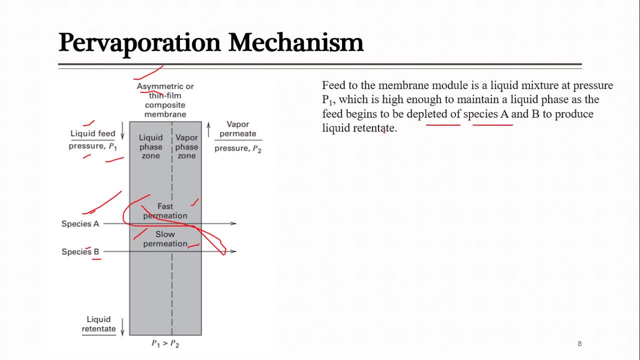 of the B will get diffused through this membrane And the mean some components are feed is actually depleted mean some component has been removed from this feed. they have permeated through the membrane, So still it exist in the form of liquid when it is leaving this feed side. 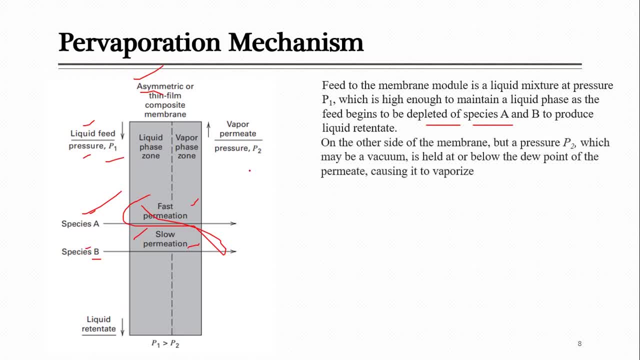 as a retentate. On the other side of membrane you have pressure, P2, and which is most of the vacuum. you apply here the vacuum, And I already told you that the purpose of vacuum is to reduce the ambient, and when you are reducing ambient pressure, you are converting the phase from liquid to 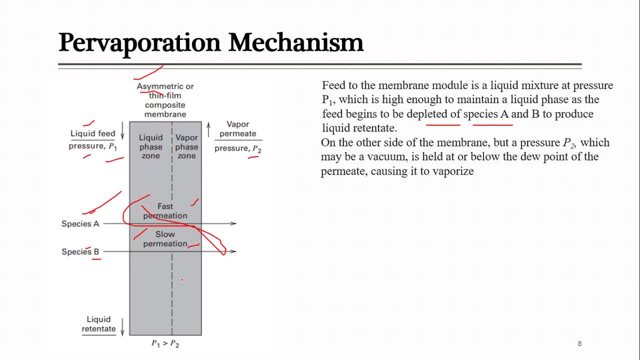 vapor Here in this. this is the membrane module In this. he has just separated this in the two parts, So let us talk about this somehow 1 or 2 minute later. Composite membrane are used here and the reason of using composite. 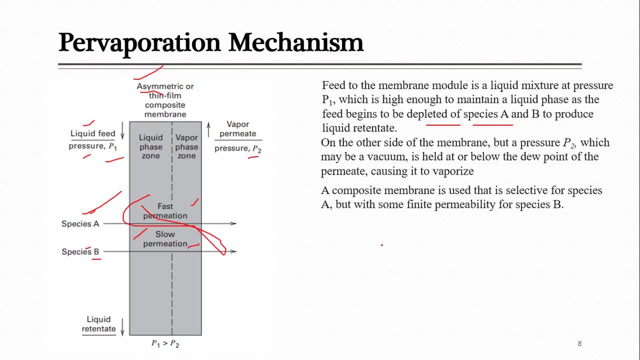 membrane already told you that- to support high pressure. So this composite membrane is used, which is selective for the species A but for somehow finite permeability for species B. I mean small amount of B can also pass through this main composite membrane And reason is to use this membrane to be- I mean to operate this process at high pressure. 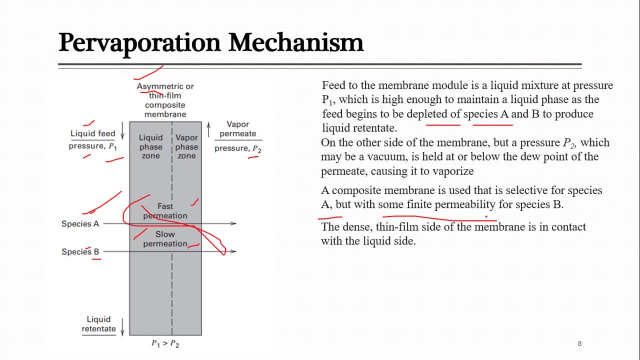 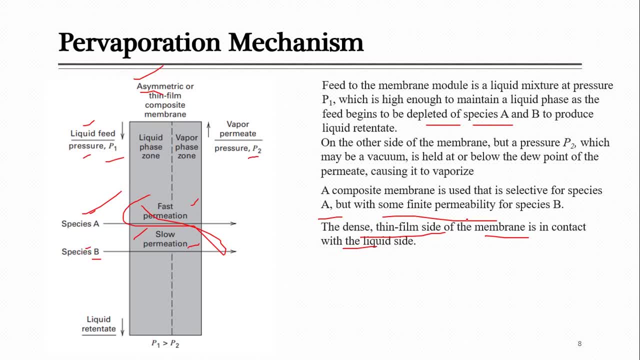 these membranes. So this is important when you are placing these membranes, So as this membrane is combination of porous and non-porous membranes, So dense membrane, film side, which is major, means separation layer or active layer that should be placed on the liquid. 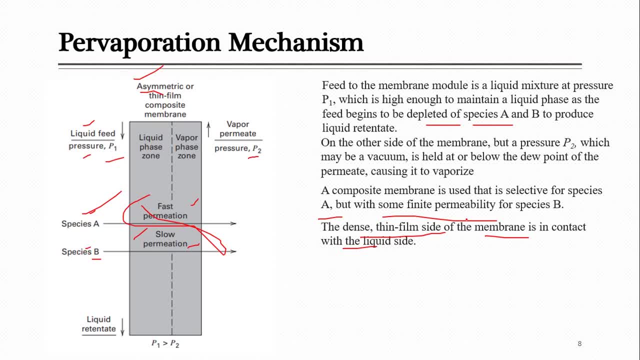 side, because through your liquid something has to diffuse and then pass to the other side of the membrane. So this active layer should be on that side from where you want to make separation. On the other side only those component exist which are actually separated. 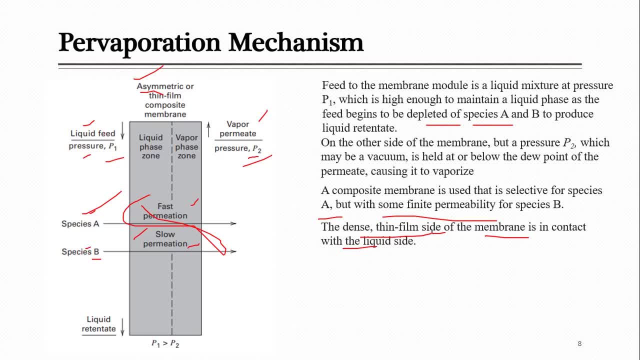 but on feed side there will be a mixture. So this dense thin film side should be on that side, and this is same for even RO and gas separation. when you are using, You use this thin film like dense membrane, which is active layer. this is usually on feed side. 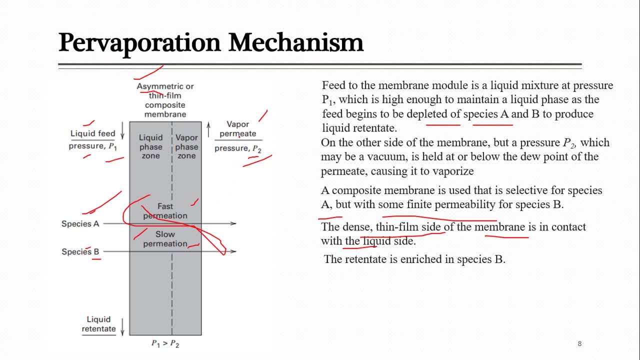 At the end of the day, when mean permeate. permeate will be like: contain more amount of A and retentate will contain more amount of B. B or B species mean large amount. The vapor phase may exist here. mean on the permeate. 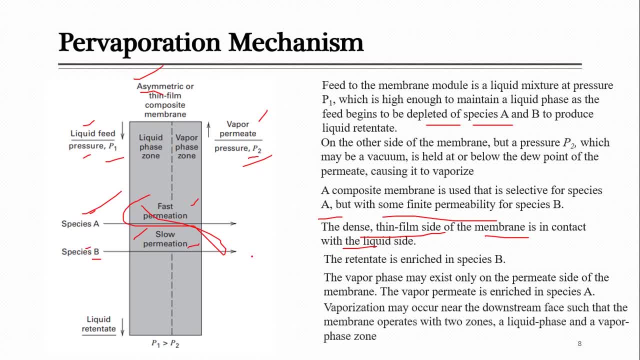 side, and that is mean usually enriched in A. This vaporization mean may occur even during the passage through the membrane mean. there the downstream phase. downstream mean: this is upstream from where this diffusion is starting. on the other side, This is downstream side from where these. 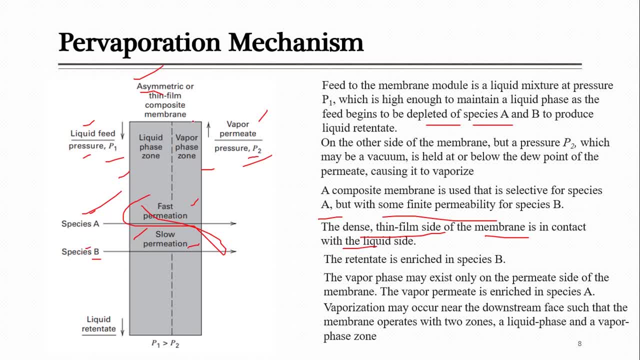 Species. A molecule will be leaving the membrane- This is downstream and other upstream, from where it is entering, So through this membrane. when this A, which is in the form of liquid, this diffuse through the membrane while passing through the membrane, even inside membrane. 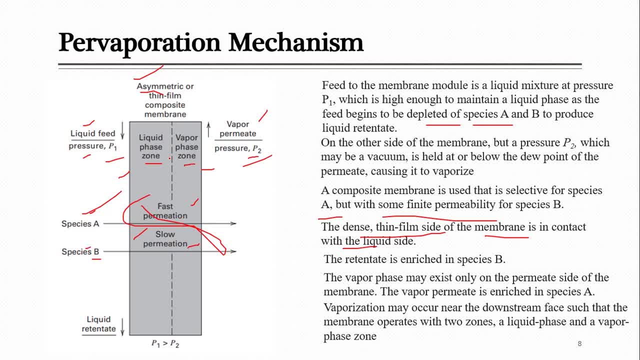 there are two zones: liquid phase zone and the vapor phase zone. What does this mean? that through this membrane, when it will pass, it will exist in the form of liquid up to some extent. 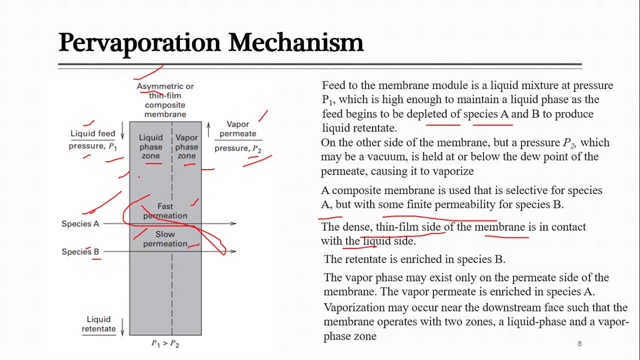 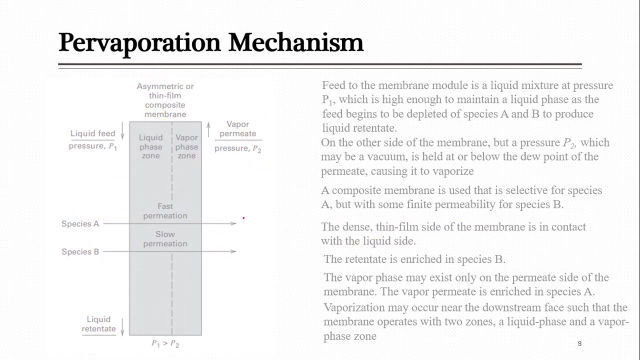 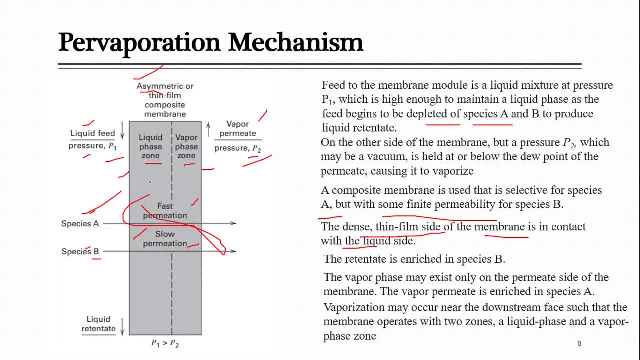 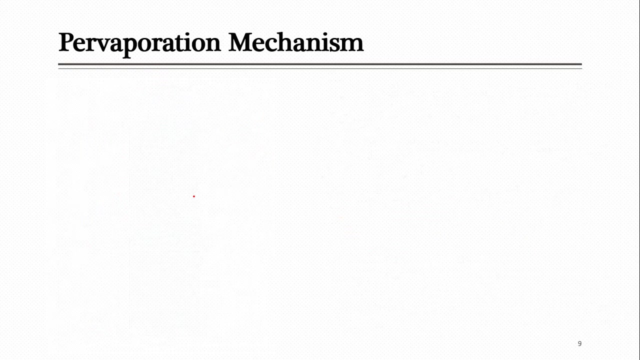 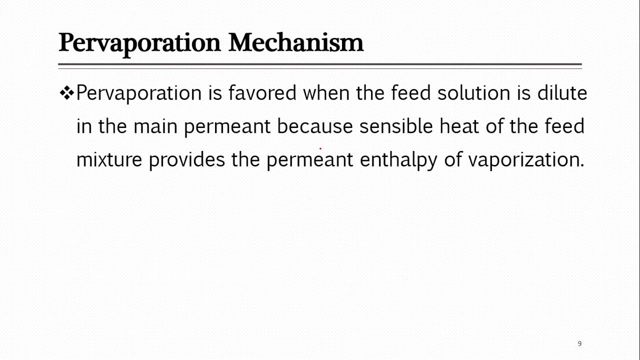 which which you want to separate. So in that case, if feed is rich in the main permeant, 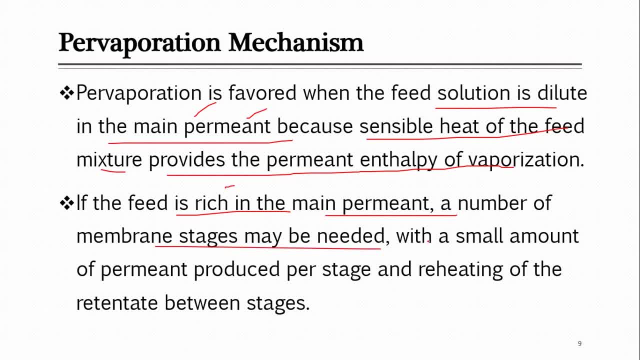 it is present in the large amount, then number of membrane stages may be needed, more than one stage. you will need why? because in each stage small amount will be permeated, because energy needed for this heat of vaporization is coming from the feed and you can provide. 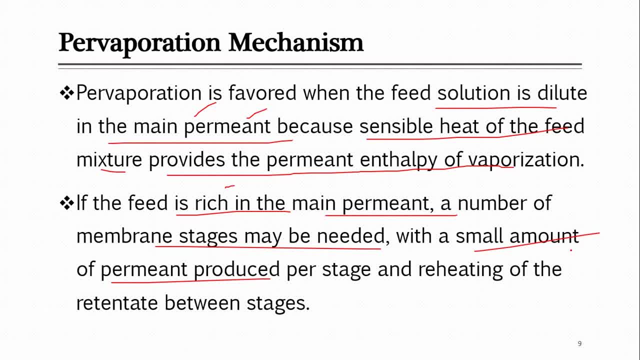 somehow some amount of feed, but not for the all components which you want to separate. So you will just pass it to the other stage. but before passing it to the other stage, definitely we will need some heating, So reheating of the retentate between stages will be needed. 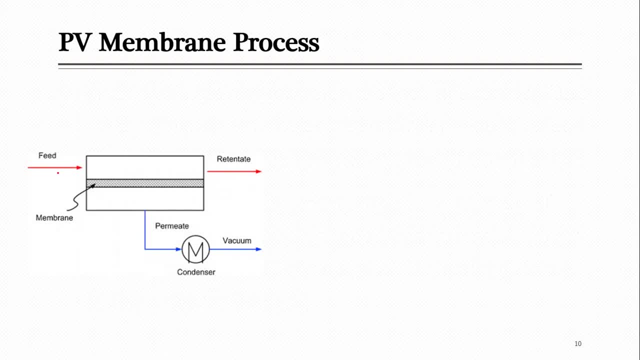 So just look at this diagram here. you can see this is the one stage phenomena in which you are entering the feed through this membrane and this is the membrane in this membrane module. on the other side, you have applied the vacuum. you can see this. I mean this side. 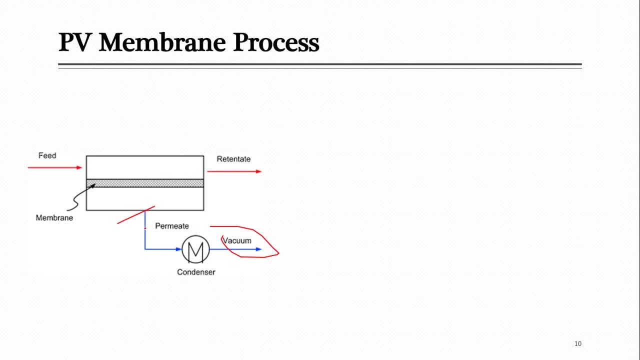 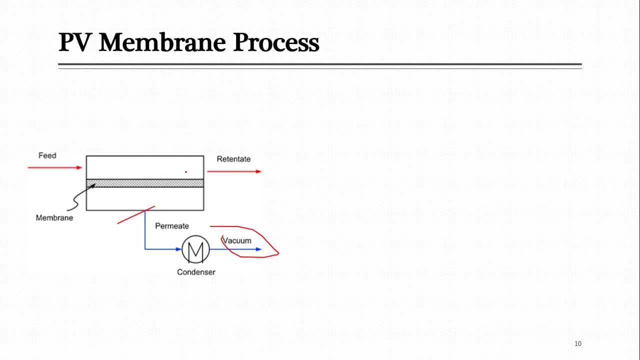 vacuum is applied And when you are applying the vacuum on this line, So this vacuum also effect this part and, due to this effect, mean more component can get separated. So retentate leaves. and this is just one phase. but if you are using more than one phases, So what will happen? your feed comes. 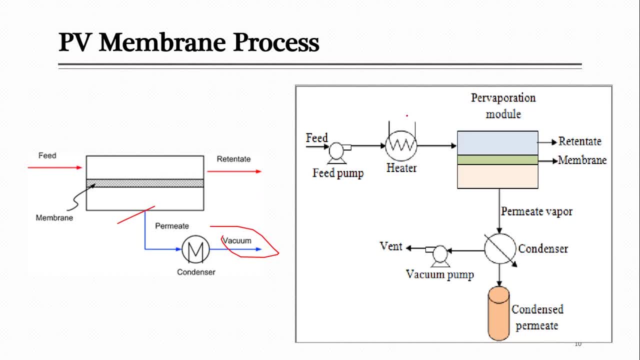 you heat it up and sometime we heat it up because we provide the heat of vaporization later on needed while passing. 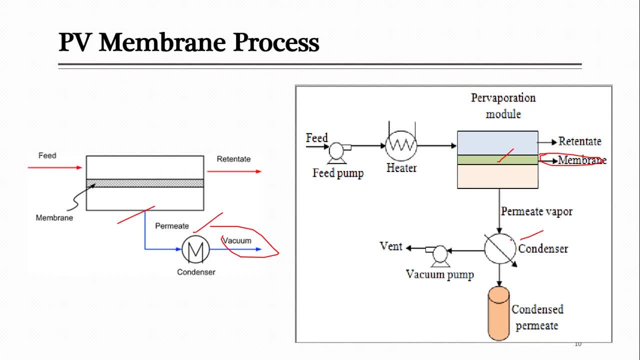 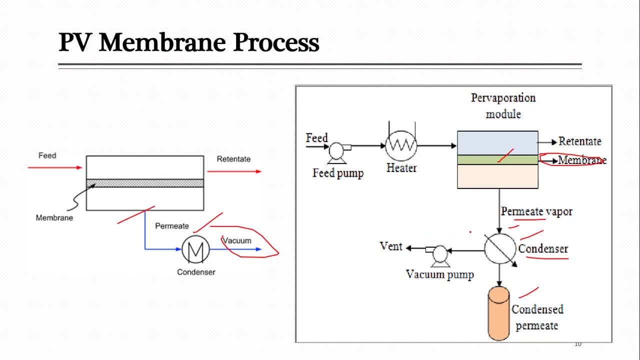 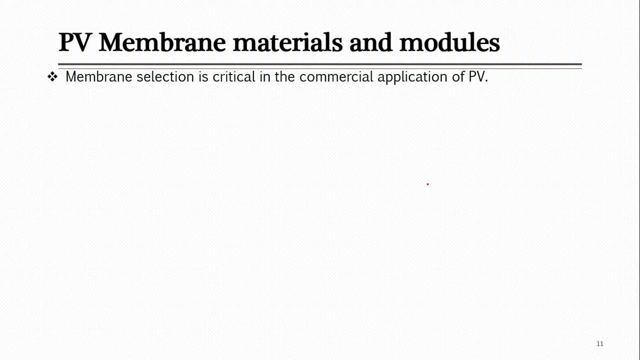 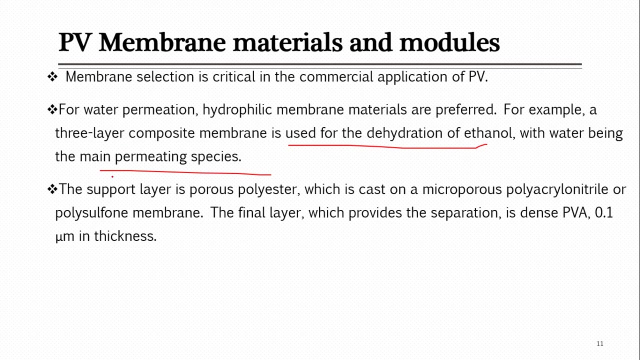 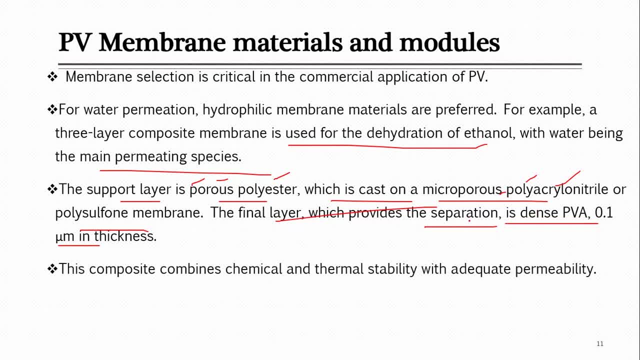 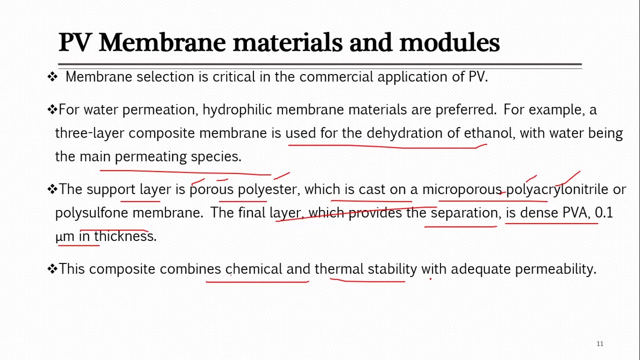 will get converted to the vapor. The composite combines here mean chemical and thermal stability for adequate permeability. This composite mean which you use so that combines chemical and thermal stability here as well, as they provide the support Chemical mean it should not react with, like your layer which you are using on the top. It should not be reactive. 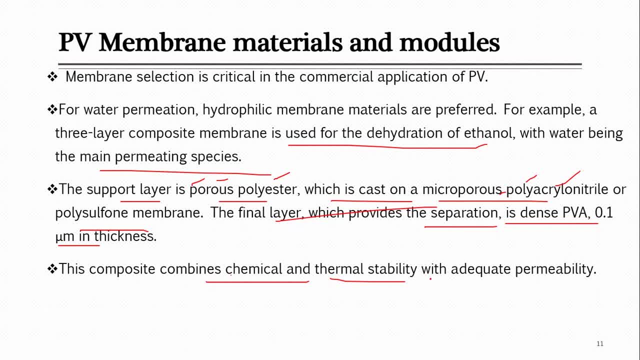 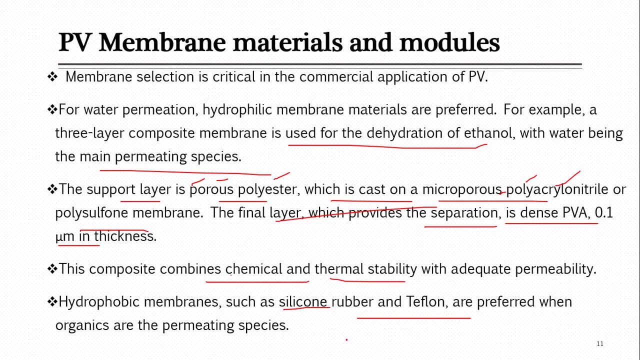 even with the hydrocarbon or chemical which you are separating, It should only be used for the separation or mean it allow only water to pass through this. Hydrophobic membranes such as silicon, rubber and Teflon are preferred for mean application when organics are the permeating species. Mean in that case, then those this silicon. 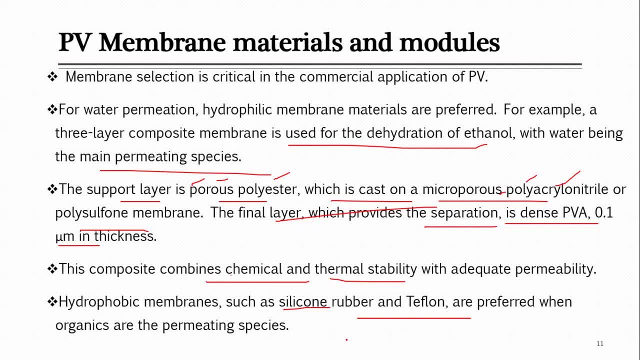 rubber or Teflon. they do not attract water, They attract air. So they are not easily the hydrocarbon or other components. and this is not hydrophilic, It is hydrophobic. It will not attract the water. So water is not the major permeating. 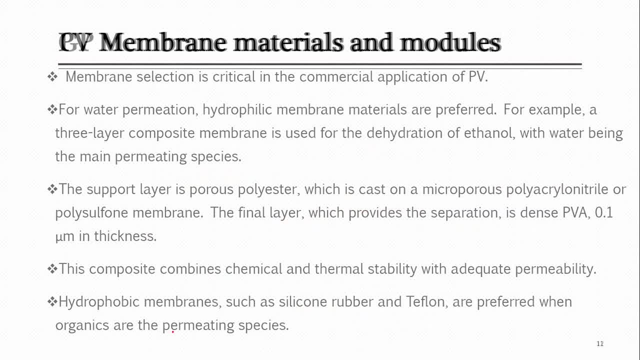 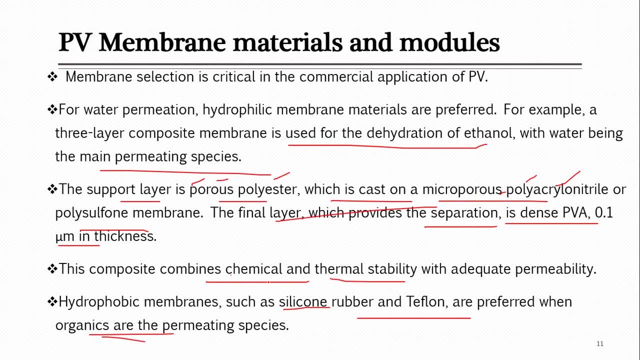 species. In that case, other component like organics, will be here, major permeating species. This was all about the materials which are used. So in this case you can see that actually here the material you have to select based on the separation which you want to take, either. 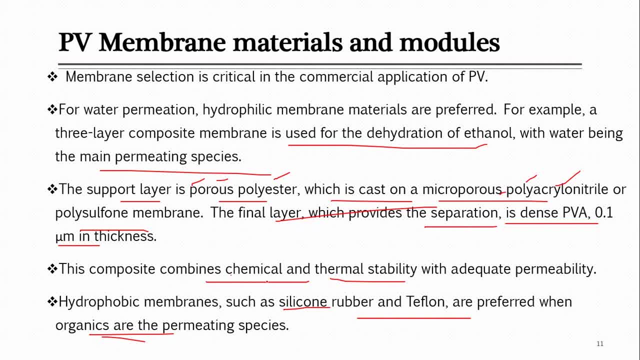 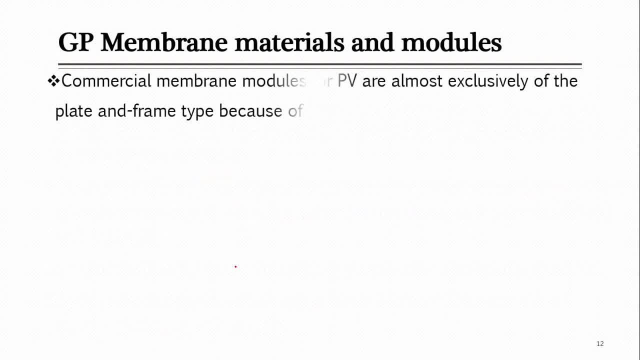 you want to remove the water or the other material. So in this case you can see that actually, here the material you have to select based on other organics from the membrane or permeate species, which is your permeate species. then, based on that, you have to make this selection. 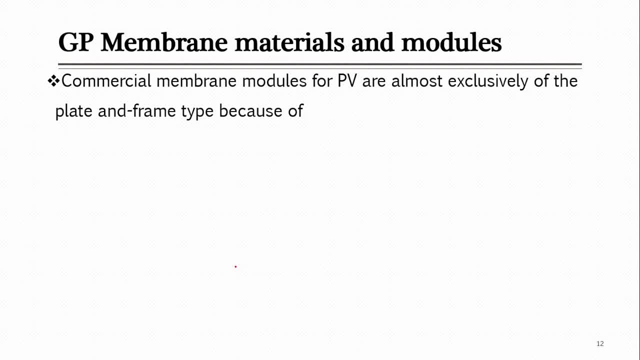 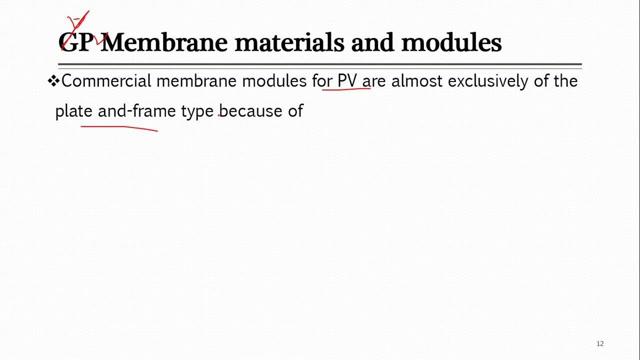 Regarding modules, so mostly commercial membrane modules for this pervaporation. So this is Vp pervaporation. This is not like Gp, This is not gas permeation, It is pervaporation. So for this I mean pervaporation, And there are the comment that if the pervaporation neverинаectere, So is the pervaporation ever. 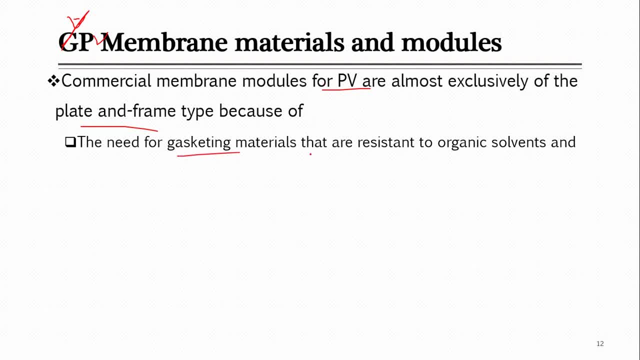 in the pervaporation or even in the pervaporation sit. So mostly used plate and frame type modules and there are the certain reasons for this module usage. So first reason is: like you need here gas getting material and those material which you are using for gas getting, they should be resistant to the organic solvent. So, as you know that here in pervaporation, we are using the vacuum and in order to like, maintain that vacuum definitely, and also use the pervaporation material which is already there, which has frequent능, heuristic, which which exist in 있게 Now, from here we do some. 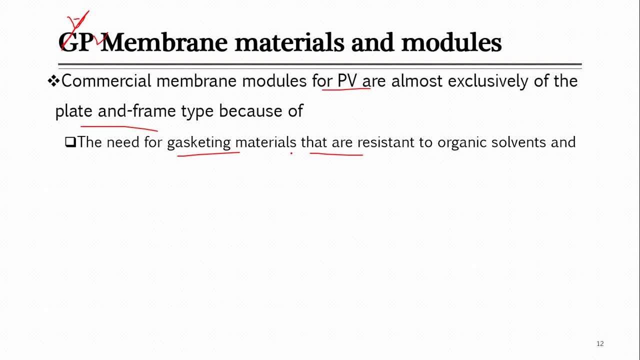 definitely you will be needing gasketing and gaskets. you know that these are just like structure, which are used to avoid some leakage. So, in order to avoid this leakage of pressure, to avoid this, I mean to maintain the vacuum- So you will be needing gasketing inside. 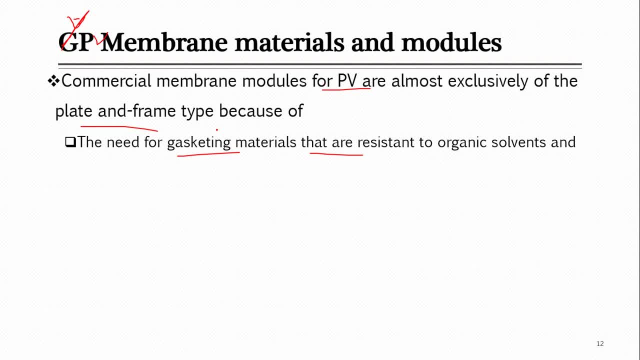 these equipments, I mean these membrane separating equipments and for that purpose plate and frame can be easily gasketed. So from the start, when we looked at this, I mean various module hollow fiber spiral wound like this plate and frame. So, plate and frame, there are the plates. 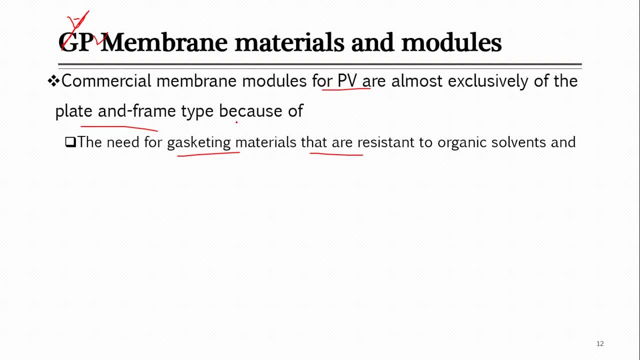 and inside that these membrane are in the form of frame So you can easily gasket those, you can easily apply those. I mean just gasketing materials and they, due to this these are preferred like plate and frame. So, compared to this, will be difficult to maintain that vacuum in the form of like spiral wound or 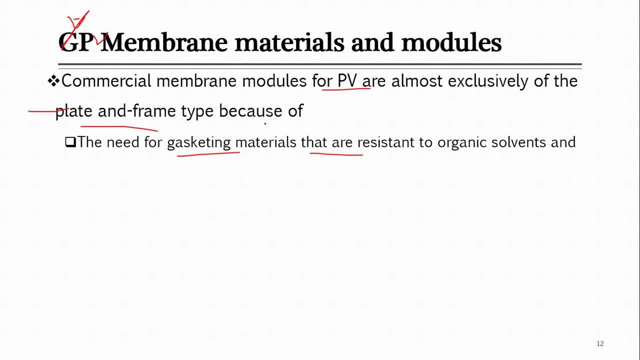 hollow fiber. just consider that when you will apply the vacuum, those fiber, I mean, can't maybe maintain that vacuum as well. the other spiral wound module inside that vacuum is difficult to maintain as compared to this plate and frame. Then this material which you are using for 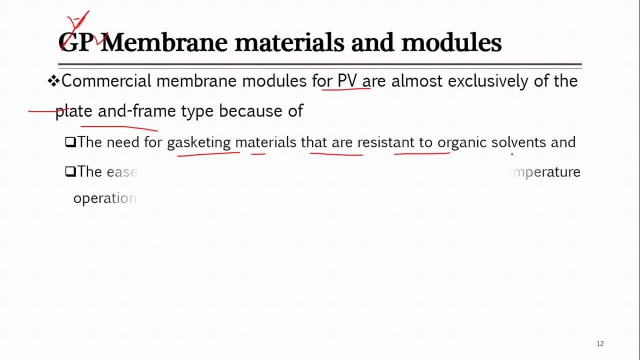 gaskets that should be resistant to the organic solvent it is necessary, Then. the other main advantage of this plate and frame is the ease of providing heat exchange for vibration and high temperature operation When you are using this plate and frame in these techniques. if you have. 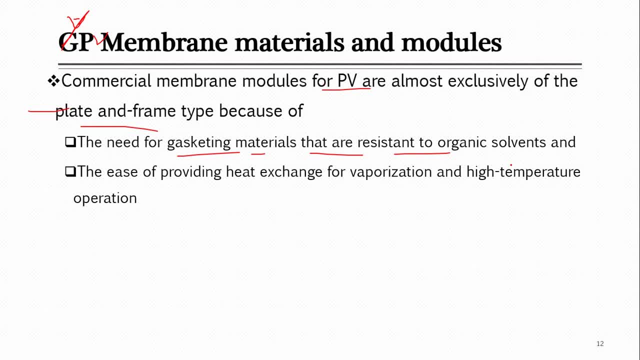 to provide the heat inside this. for this vibration I mean one. we are reducing the temperature, although at the same time in some application maybe you need to provide the extra heat during this phenomena. So in plate and frame I mean easy to provide this heat. their structure are such that inside those, 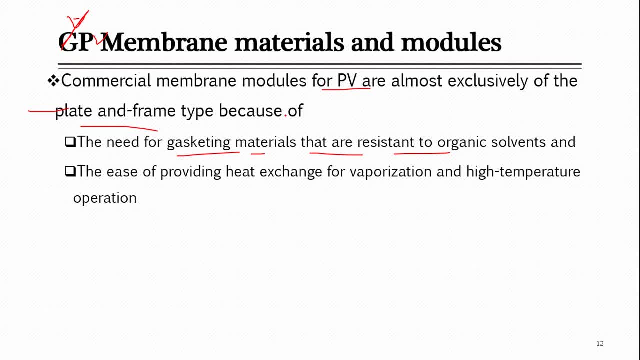 modules. It is easy to provide the heat just for this purpose. go back to those modules and look at those. when you will look at the plate and frame module, So they are structured somehow easily, there are the like plates and membranes are installed inside them. So there, maybe you can. 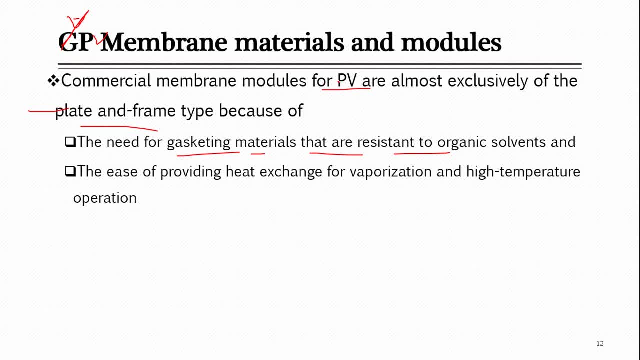 dedicate some parts for heating, So this is very easy to provide that heat. So for this purpose- I heating purpose. as compared to this, again in spiral wound and in hollow fiber membrane, it is difficult to provide heating inside the membrane Most of the time. when you look at 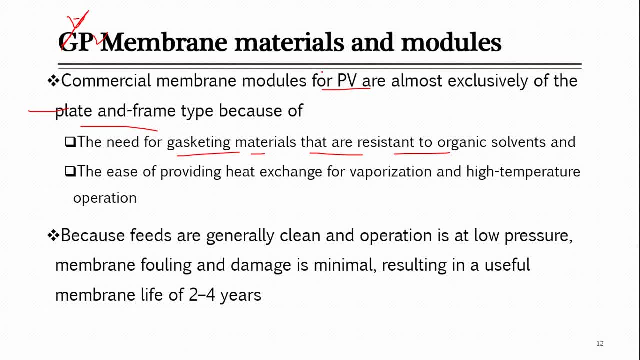 this I mean PV power evaporation, so your feed are generally clean because they are coming from the reactors. mostly these hydrocarbon are produced in the reactors and they contain water, so you want to separate them, or even they are closely boiling hydrocarbon mixture. so they are these. 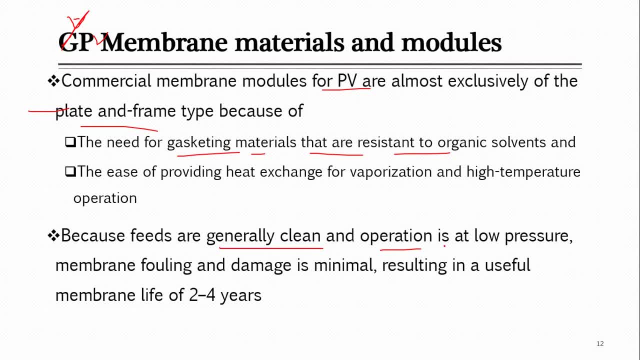 are usually the clean feed. these are not like the gases which can contain particle. these are not like the water which contains some, a lot of main impurities. so here these are usually the clean. due to this, most of the time you don't have any pretreatment unit in such per evaporation. 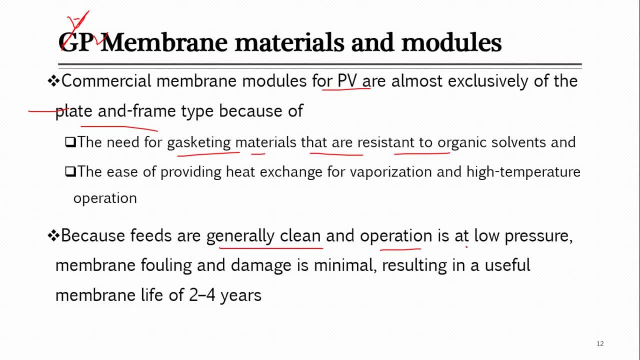 membrane. so because you are operating them as well at the local level Pressure as compared to the other. I have told you already that they are operated at the low pressure as compared to the reverse osmosis and gas separation. so due to all these advantage, clean. 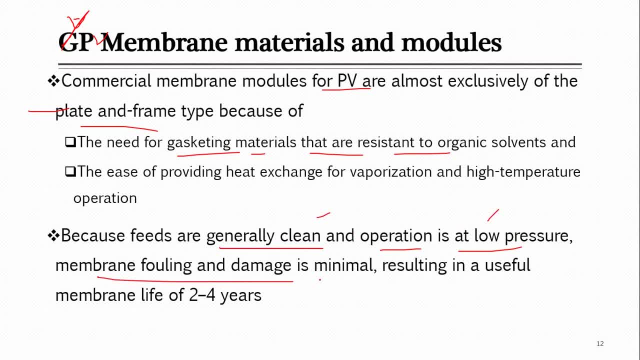 feed operation at low pressure. so membrane fouling and damage is minimal in these type of membranes. so this membrane can get damage due to high pressure as well, due to the fouling, due to accumulation of various other main components on its surface. so that is very low pressure. 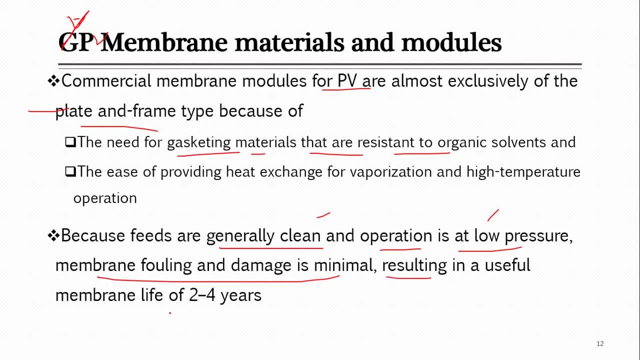 So in these kind of membrane which are used for per evaporation, due to this they can be used for up to 2 to 4 years. Most of the time, by the way, membranes you have to mean replace membrane, like after one to two years. I mean sometimes you don't replace them, you go for the cleaning and until unless 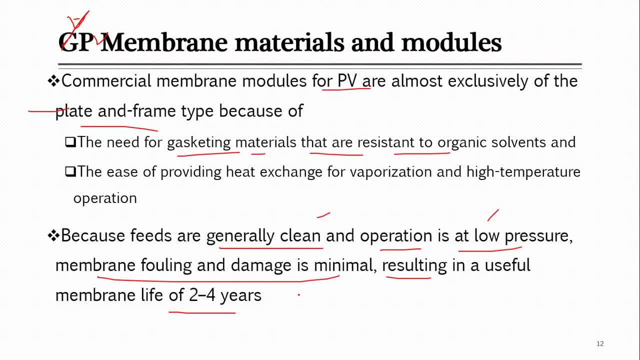 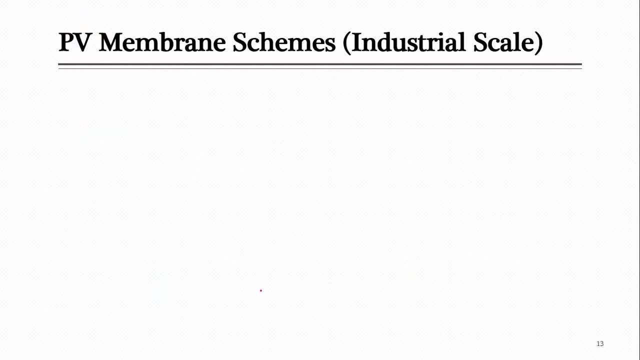 they are not completely blocked or they are not providing sufficient permeation. so then you go for their replacing. But this is, I mean, large time to clean: One to two to four years. Let's look at some per evaporation membrane scheme which are used on industrial scale. 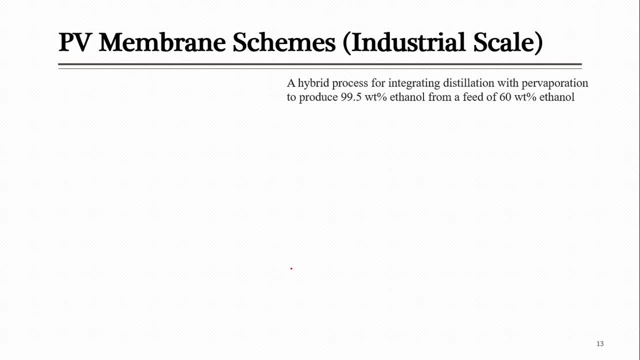 so sometimes they are used separately. sometimes they are used in the combination of various other techniques, Like here. there is one used for the. I mean hybrid process, hybrid process for integrating distillation along with per evaporation. it is mean there will be distillation as well. 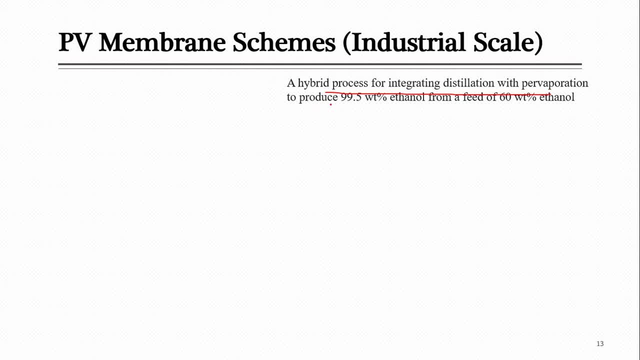 as per evaporation. So to produce 99.4 percent- Just say that Esto bourbon, in tablespoon, I think- which we till 24.5 percent ethanol from a feed which contained actually 90 weight, sorry, 68 percent ethanol. So your feed contain only 60 percent ethanol and you want to purify it to the 99.5 percent. 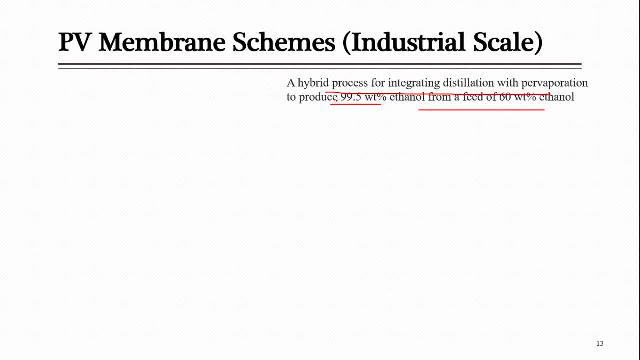 ethanol. actually it contains water. 40 percent water is in the feed and you want to remove to it that water and finally you want to get 99.5 percent ethanol. So in this technique, the common technique which is used on industrial skill, that was distillation. 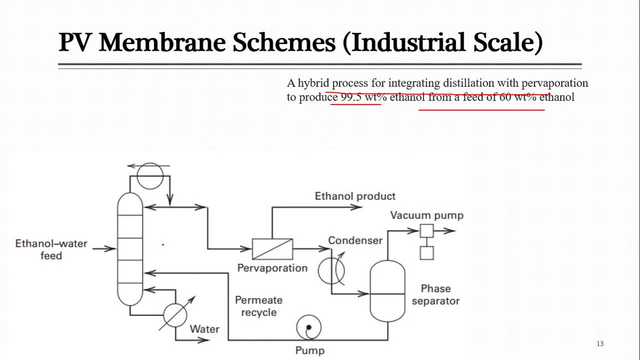 and with the help of distillation, the per evaporation nuance distillation. you can see this first part of this, I mean PFD. So in this part ethanol water feed enter to this. I mean distillation column. and then there is condenser and reboiler along with this. 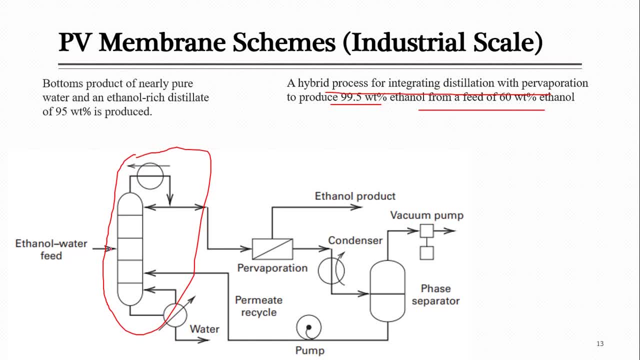 And at the end of this I mean when you look at the products, bottom product is purely water. At the bottom, from this reboiler you are getting the water, So that is pure water. you have separated some water And from the top definitely you will be looking for the lighter component. 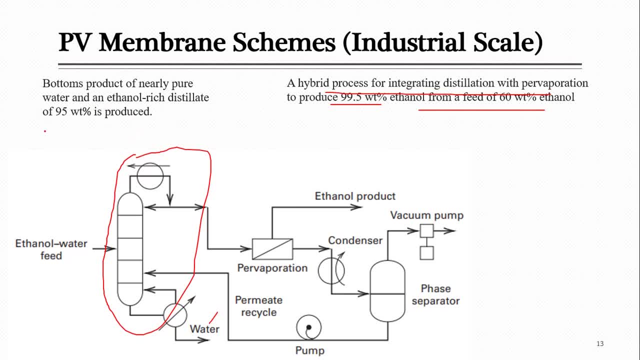 ethanol to be- I mean obtained as your product. Then you are looking for the product of purity 99.58 percent, But here its purity is 95.8 percent. from this, And even if you install these- I mean equipment of distillation- maximum what you can reach is 99.58 percent ethanol water. I mean. 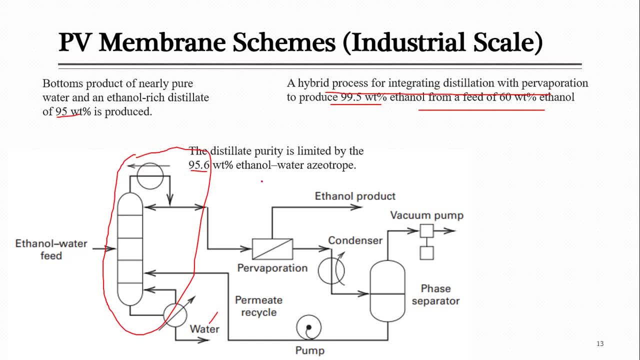 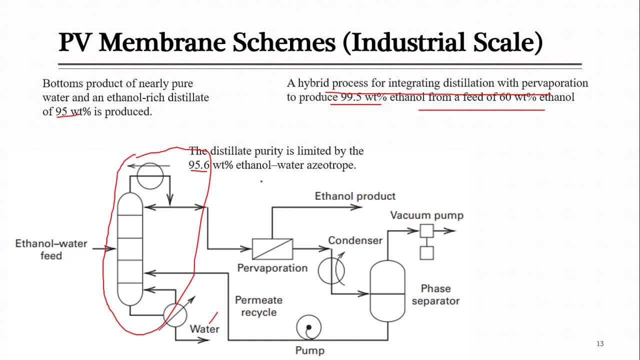 you want to go for further separation with the help of distillation, maximum possible is this: 95.6 weight percent main ethanol purity. Still, there will be some amount of water present with this, like almost 4.4 percent water is there. So in order to avoid this water, to remove this water, 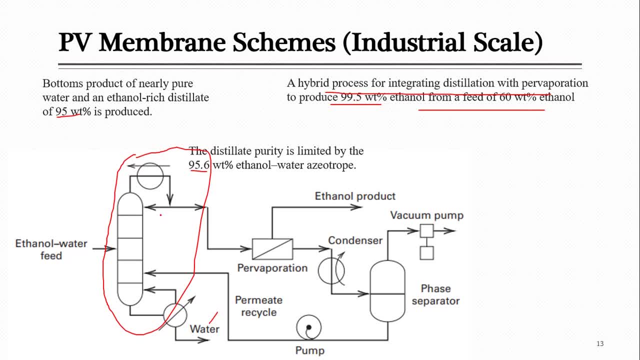 to make it purified up to 99.5 weight percent. this part is sent to this, I mean, which is mixture of water and ethanol that is sent to some membrane, that's pervaporation membrane, And this membrane is, I mean, hydrophilic, which allows water to pass through this membrane and then retentate will be. 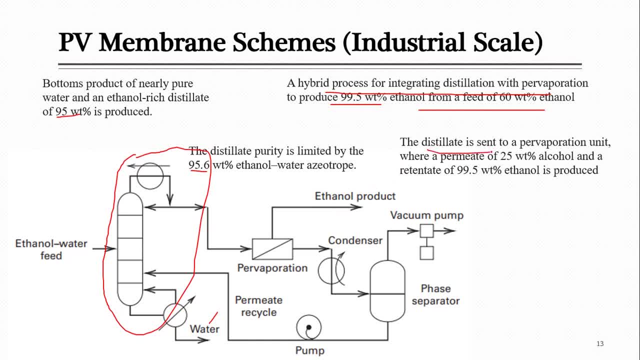 the ethanol. So when it pass through this membrane the distillate is sent to the pervaporation unit and your permeate is 25 weight percent alcohol permeate- Majorly water will pass and still through this membrane some alcohol is lost and that's overall composition. is there 25 weight? 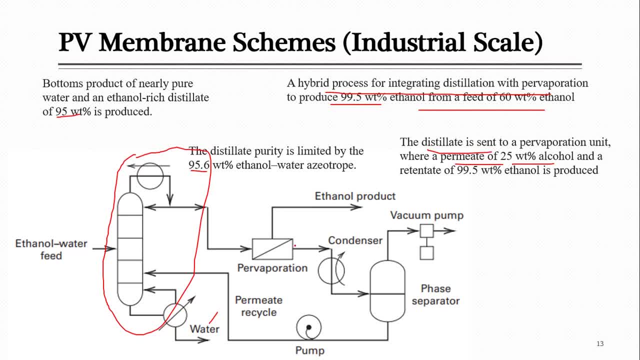 percent alcohol And 75 percent will be definitely water, while the retentate side is 99.9- sorry, 99.5 percent pure ethanol, which was your requirement. So, with the help of this membrane, you can achieve this separation. Now, looking at this permeate, because this contain, this is not only water, this contains. 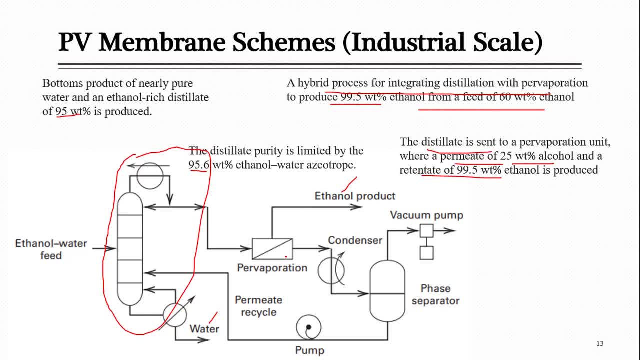 sufficiently large amount of- I mean this ethanol- 25 weight percent ethanol. So what you will do, this will be in the form of air vapor, So you just condense these vapors and with the help of this condensation, then you bring it. 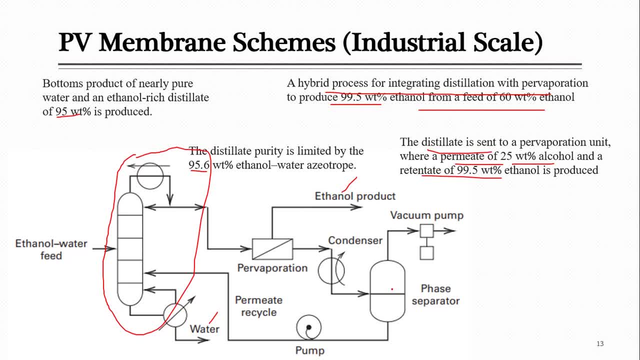 to some phase separator. In that I mean phase separator. actuallythis mean liquid and vapor. all that. this is not definitely complete condensation. somehow some part of this is condensed and some don't condense. So here phase separation takes place. the component which is in the form of vapor, they are just separated form. 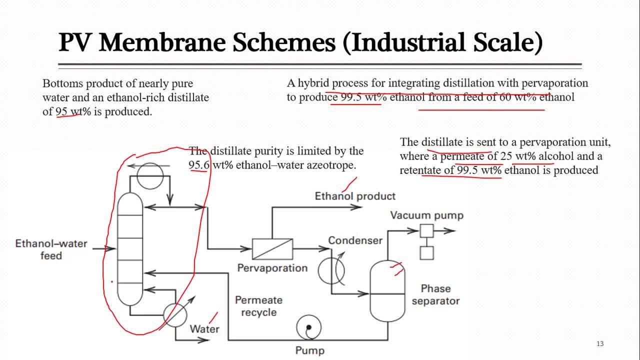 air and other, which is in the form of liquid. they are pumped back to this main distillation unit because you do not want to waste this sufficiently large amount of alcohol. So inside this here you are applying the vacuums. this vacuum is actually applied for this pervaporation. 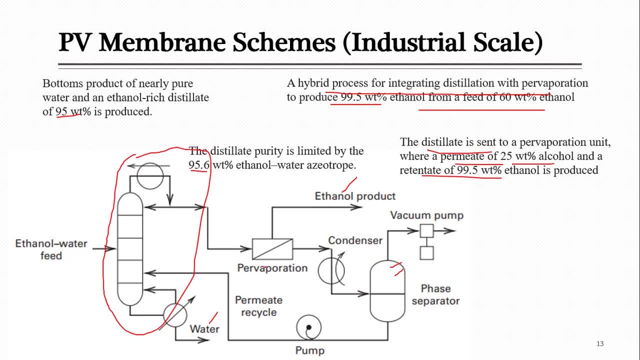 through this line, through this equipment here, when there is a vacuum- So here I mean separation through vacuum- will take place in this pervaporation, So in this example. actually, the purpose here is to separate this water and ethanol, and which cannot be separated with the help of this distillation. at the end you have to go. 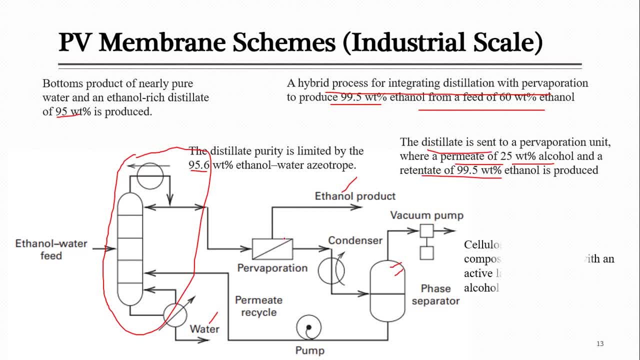 for this integration with PV membranes. Here the membrane uses cellulose acetate based composite membrane with active layer of polyvinyl alcohol. This is two layer membrane- cellulose acetate and polyvinyl alcohol- and active layer is polyvinyl and that is attractive for water, which allows in large amount water to be produced. 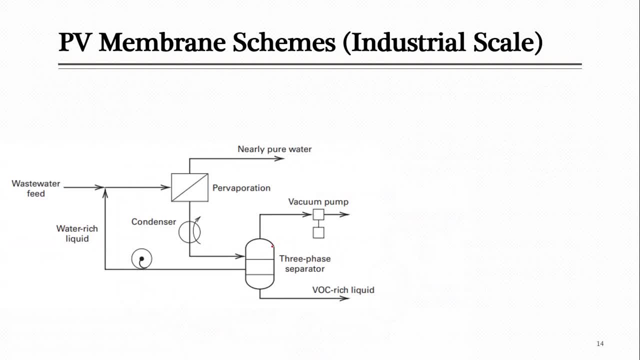 pass through, that will be hydrophilic membrane. Other main its usage is here, for example, for removal of VOC's. VOC's are volatile organic chemicals, for example toluene and trichloroethylene, benzene, xylene. a lot of these are considered under the category of this volatile organic chemical because 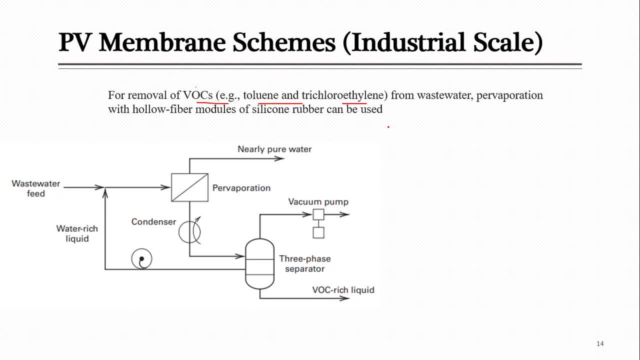 they are usually volatile at mean, even low temperature, like room temperatures From waste water. pervaporation with hollow fiber module of silicon rubber. So here you are, using silicon rubber and if you remember, from few slides back, I told you that when you want to pass these organic chemical to pass through the membrane, you use the such. 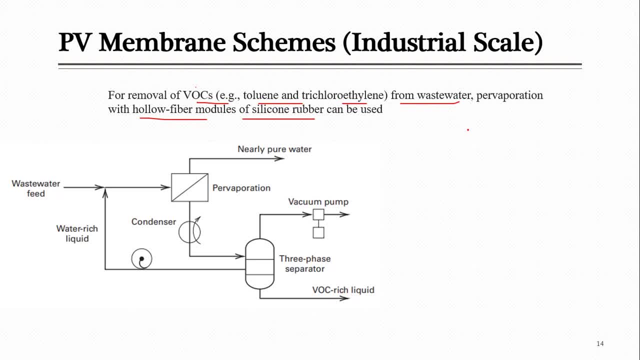 membrane like rubber or mean teflon membrane, So this will be a hydrophobic membrane. So in this membrane, when you just bring this waste water, you are just bringing it to this membrane module and inside this membrane module you are using the membrane which allows organic 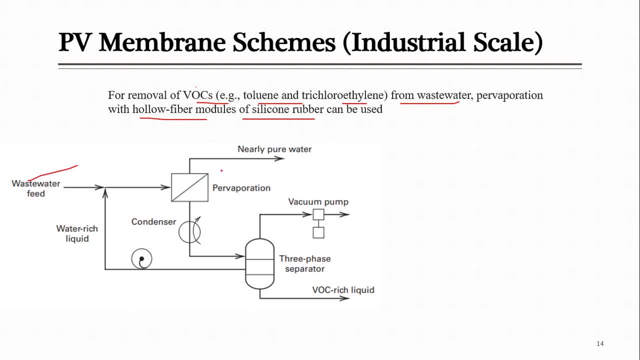 chemical actually to pass through and they can get separated. Why we are using this, by the way? because here the water is in large quantity. we do not want water to pass through this membrane. definitely we will want all those component which are in small amount to pass through this membrane. 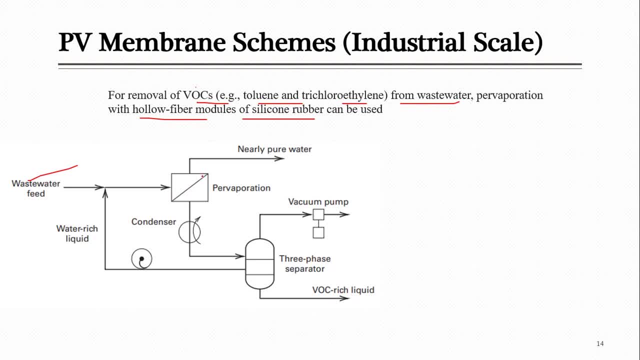 So in this, through this silicon rubber membrane, those organic chemical, volatile organic chemical pass through this membrane and they just diffuse or they just get permeated to the other side of the membrane. and this separation takes place when they are just permeated in the form of vapor. 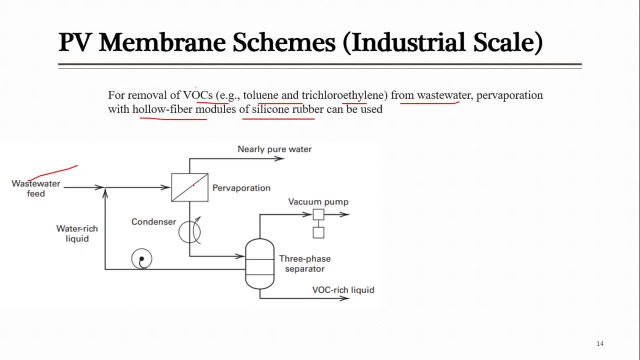 You condense them, because this membrane again will not be like 100 percent, only organic chemical permeate. some amount of water is also permeated. So you condense them and after condensation you pass it to the three phase separator. three-phase separator, Actually those separator in which there is one vapor phase and other are two liquid. 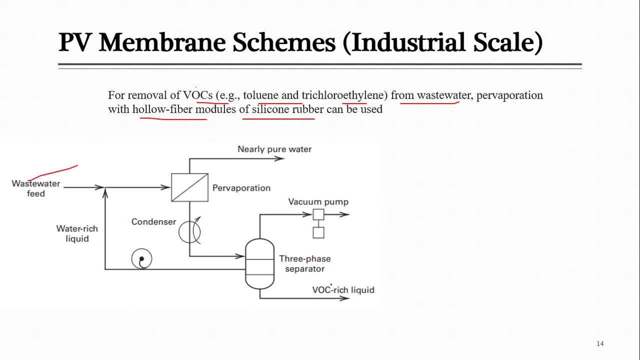 phases. and among those two liquid phases one is totally volatile, organic chemical rich mean. most of those will be volatile, while other there will be water rich liquid. So here there will be water as well as some amount of these volatile organic chemicals. So they are just sent back here in order to avoid the loss of water with the feed again. 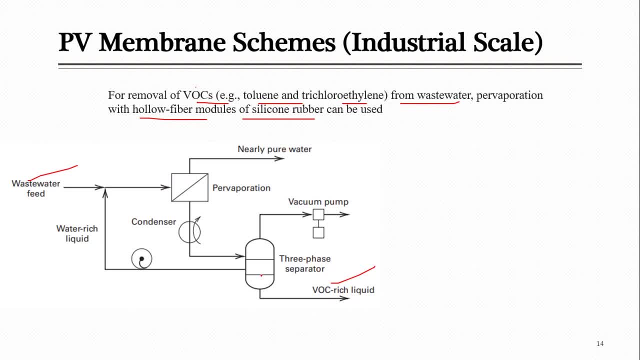 pass through the membrane and get separated, While these organic chemical, which has been separated, and they just get lost. as from here, By the way, I think here it should be- organic chemical layer should be above than this water layer, because this is usually lighter as compared to the water. 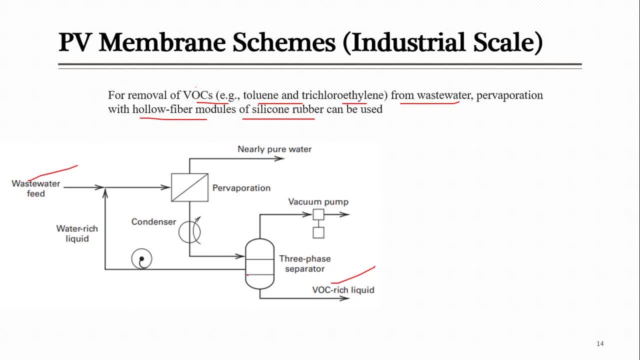 So water is the heavier and this is mainly at the bottom. So it's better to present it like: from here water And from this layer. these are organic chemical, as in industries we have like such kind of three-phase separator in which top layer is just vapor of hydrocarbon, then next layer 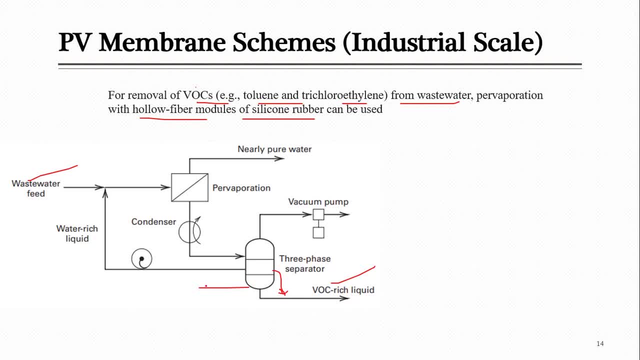 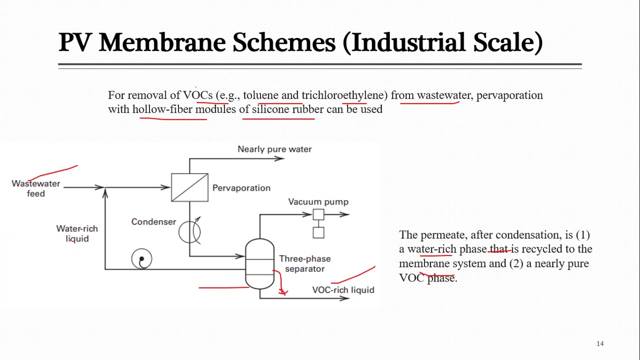 is hydrocarbon liquids and then the last layer is aqueous layer. So here permeate after condensation, mean permeate will pass through this membrane. after condensation, a water rich phase that is re recycled to the membrane system that is used, mean support water rich phase which contain large amount of water and some small amount of these organics. that's water rich layer. and 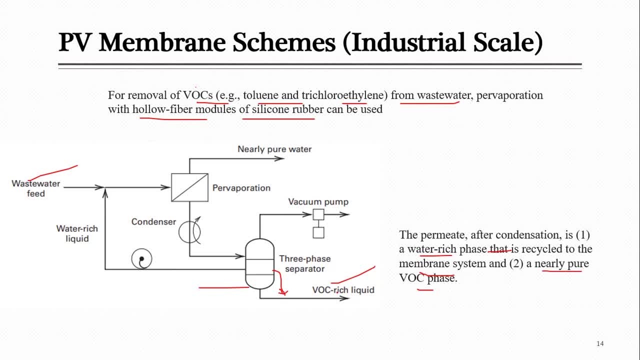 mean nearly pure volatile organic chemical phase is separated from here. So one thing here I want to mention, like he has mentioned, hollow fiber module for some application. this can be used where you can apply them, but most of the time In these pervaporation on the large scale, when you have to use most of the time, plate and frame are used. 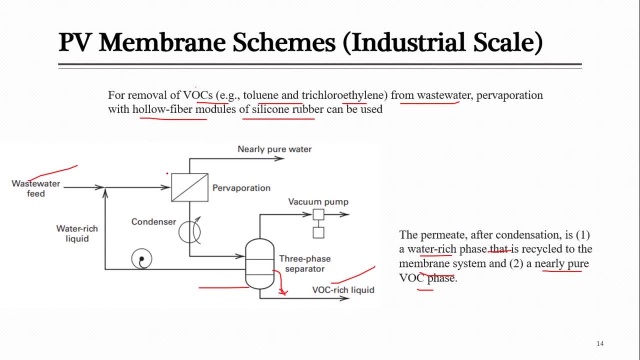 But hollow fiber are also used for some application, like in this application He has mentioned their volatile Organic chemical removal from water is taking place with the help of hollow fiber module and Retentate is pure water. retentate mean the pure water which we were looking for, which. 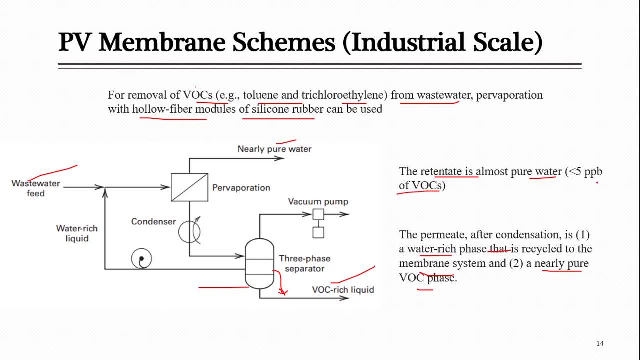 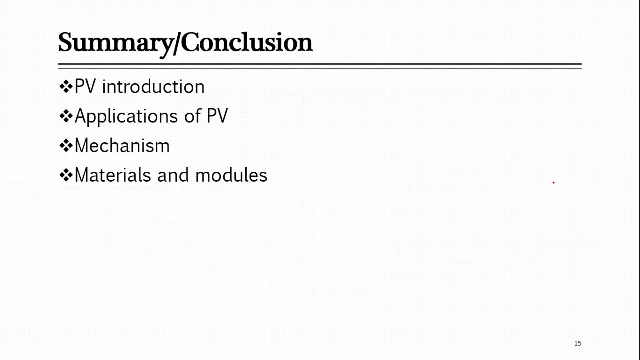 We were expecting to be pure. so that's pure. that contains Less than a five parts per billion of these volatile organic chemical way. in very small amount They will be available and that's fine for us. So that's it. in this lecture. we started with the pervaporation. What is pervaporation? 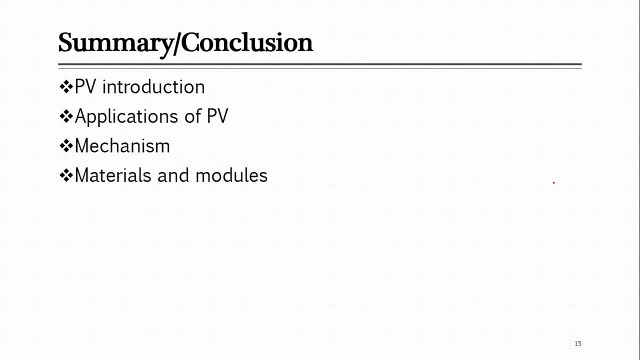 It's introduction, like pervaporation, is a combination of two words: from, from selective, and then there is evaporation and Through this membrane we have seen that when separation takes place, so after passage of permeation of the liquid species, They get converted to the vapor. on the other side, due to application of vacuum, are due to very low pressure as good. 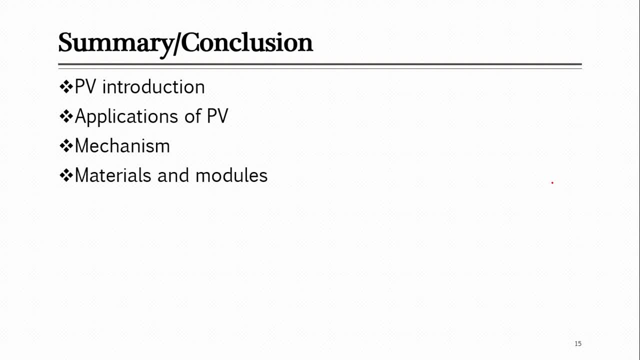 As compared to their, I mean as compared to just some ambient pressure. so Their application is mainly for removal of water from hydrocarbon, like from ethanol, ester ketones and other hydrocarbon, as well as for separation of closely boiling hydrocarbons. they are used for this, I mean. 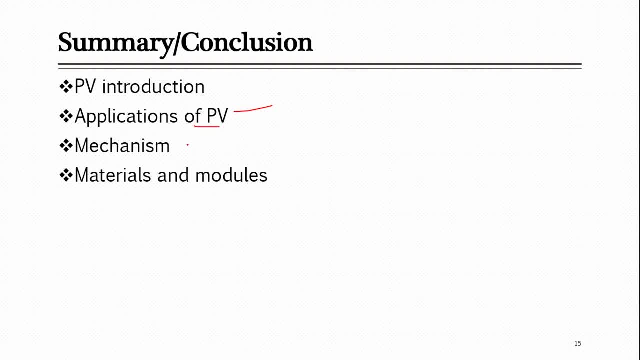 This pervaporation membranes are used and the mechanism here is: when these liquid pass through the membrane, on the other side You have a vacuum and they will get converted here. most of the time you use In asymmetric membranes. these are used because the phenomena which you are looking for, you are applying the vacuum. 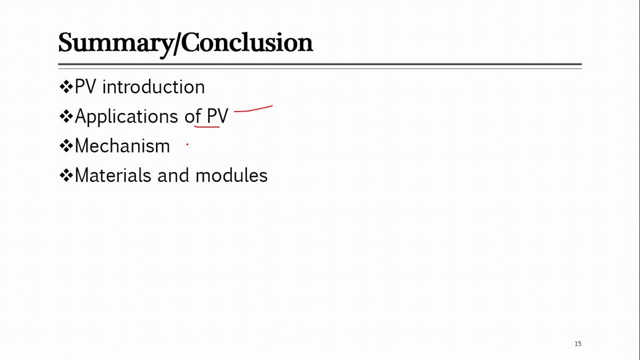 And if you apply porous membrane, then vacuum will be transferred to the other side and you can't maintain on the feed side There should be high pressure and the other side, permeate side, there will be low pressure, This vacuum. due to this you apply the dense membrane and mostly they layer. Come time, three layered membrane structures. 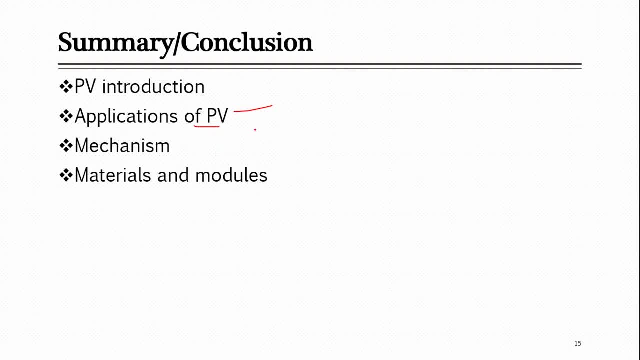 one is dense top layer, active layer, then there are two porous layers and finally, Material. material should be selected wisely based on either you want to separate the water through those system Or you want to separate hydrocarbon, and we will prefer it based the Application, like, if water is in small amount, then water should be allowed to pass through the membrane and if hydrocarbon are in small amount.